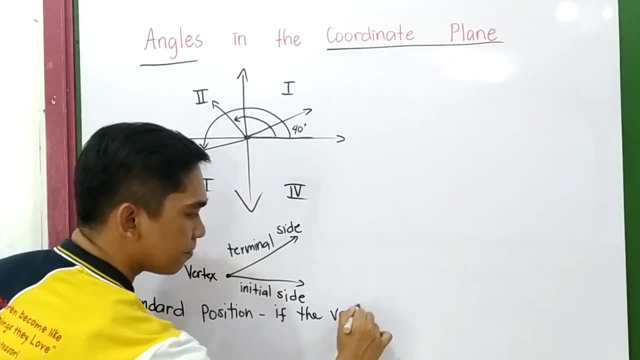 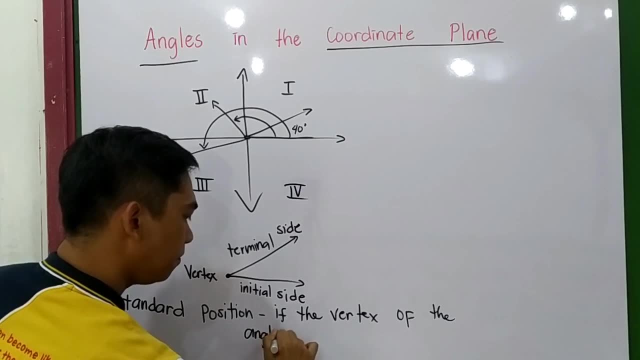 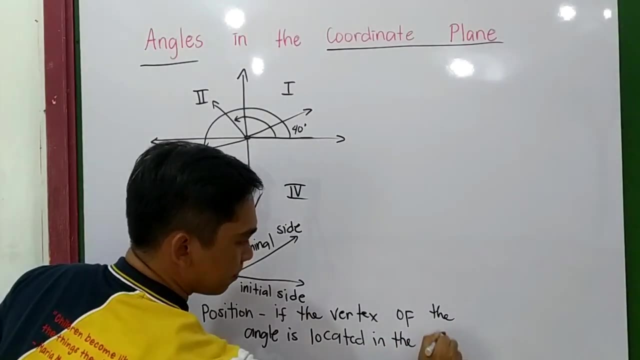 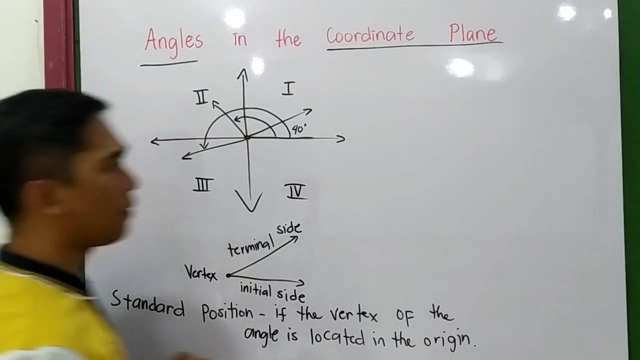 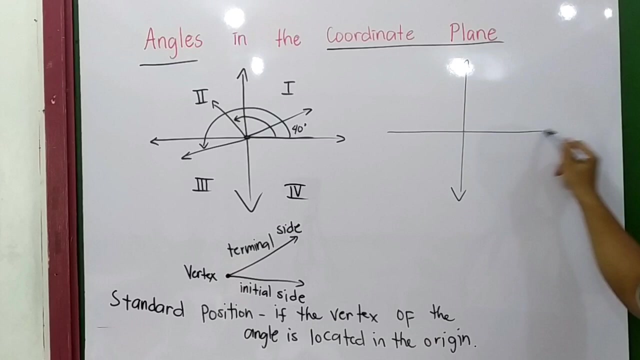 If the vertex of the angle is located in the origin- Next definition- In a partition plane from our initial side. this is our initial side, the next axis. if we take one rotation, counterclockwise rotation, is equal to 360 degrees. 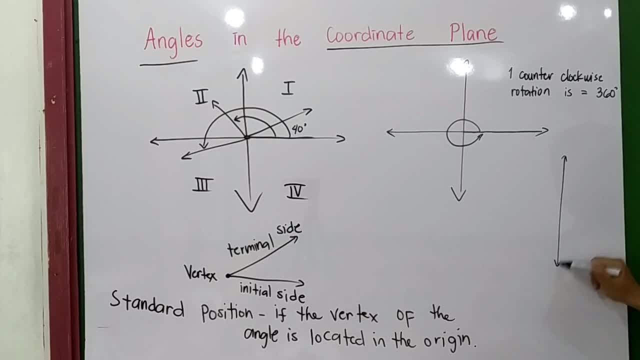 And if we have one clockwise steering, one clockwise direction, then it is equal to negative 360 degrees. So our rule: if our angle rotates in counterclockwise, therefore the angle is past here, And if the angle rotates in counter. 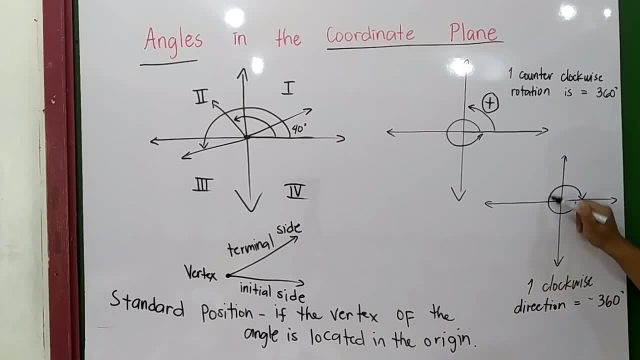 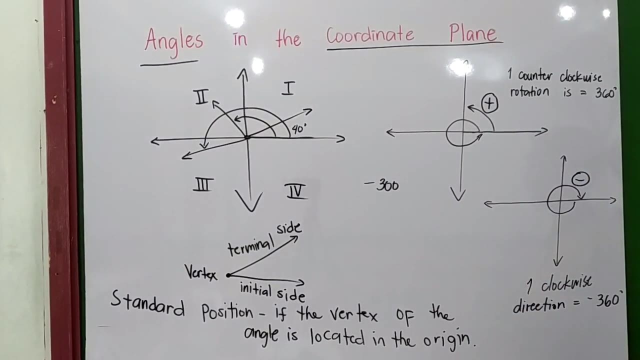 or in clockwise direction. the angle is negative. So if I am going to get negative 300, so let us graph negative 300, so we will start at the initial side, since it is negative, then we will rotate clockwise. So negative 90,. 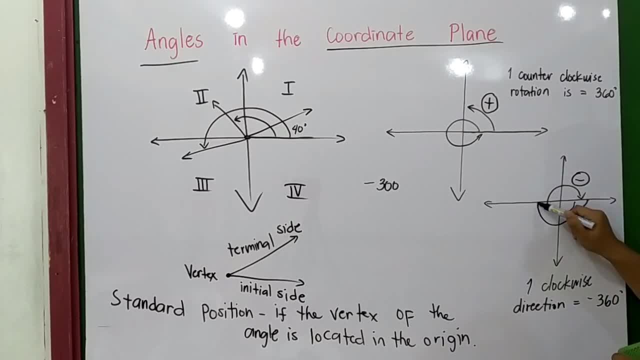 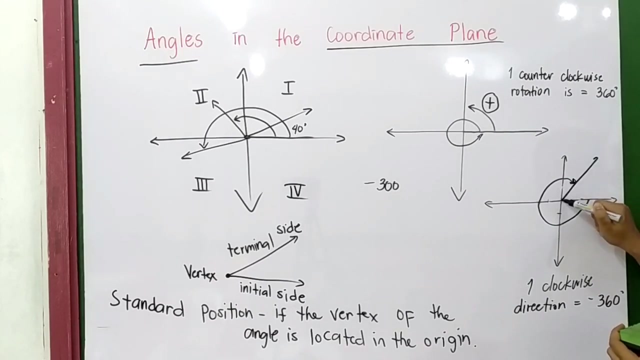 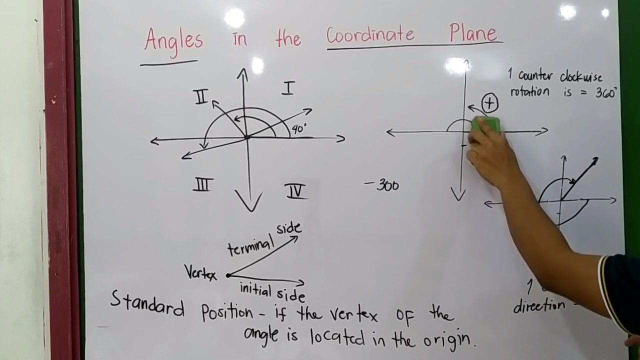 negative 180, negative 270, then I will add 30 more to get the negative 300. So plus 30.. So this is now our angle And this is the terminal side. Let's try the past game, If they ask you to find. 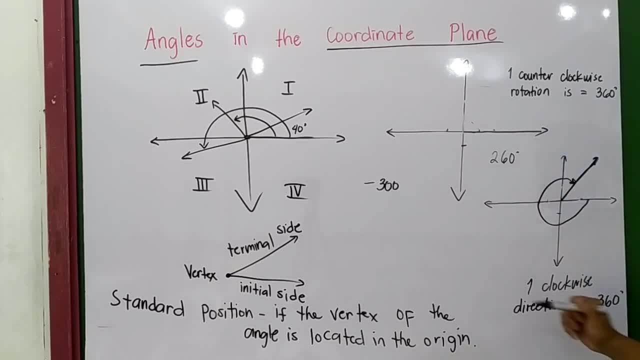 you have a negative 360 degrees. So, since this is past here, counterclockwise direction: 90, 180,. here is 270, so before 270, so 260 degrees And this is the terminal side. Get it. One rotation is equal to 360 degrees. 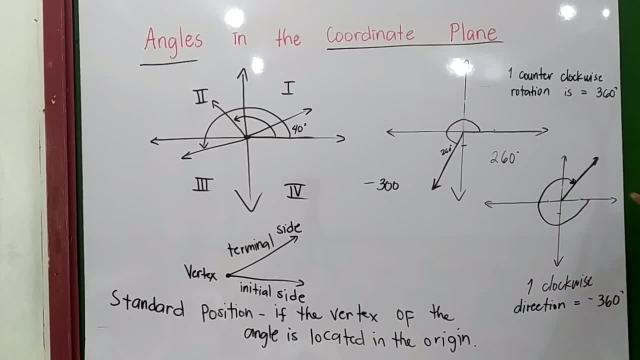 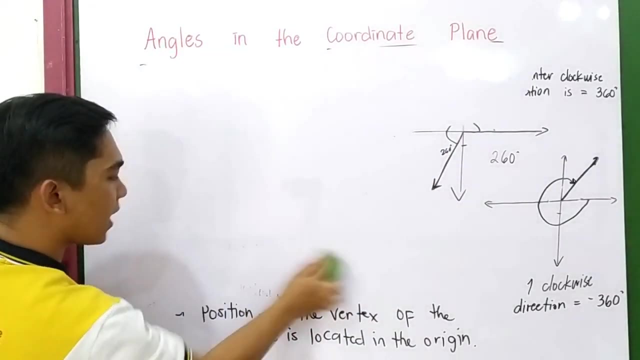 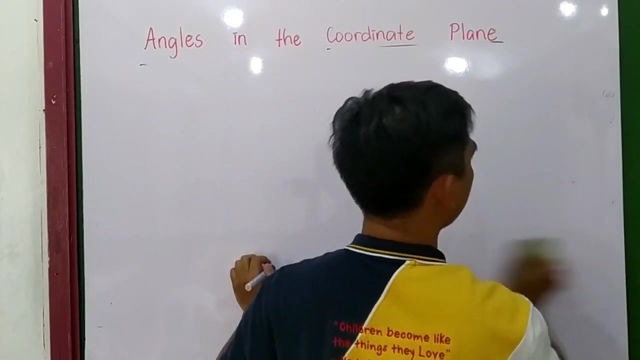 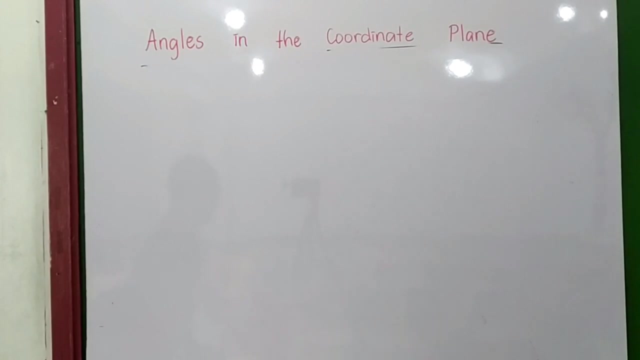 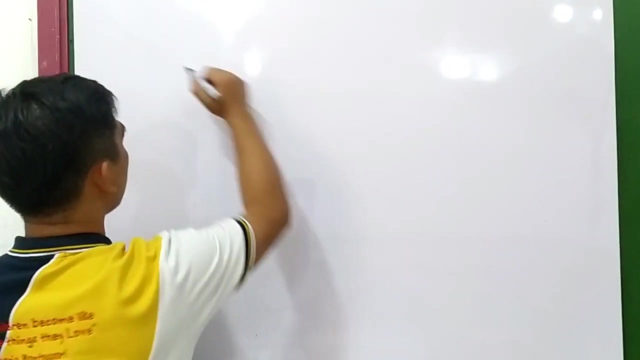 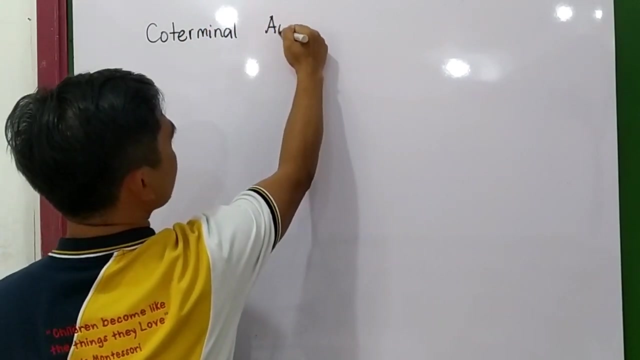 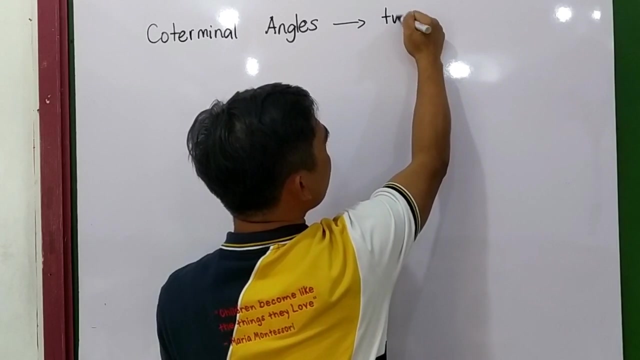 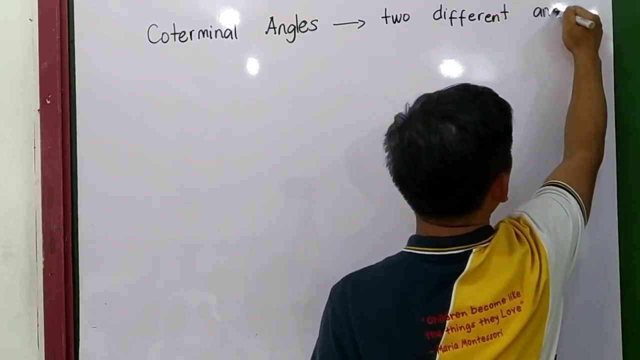 If the direction is flat-wise, therefore, it is negative 360 degrees. Let us proceed in next definition: Codeterminal side. Let us proceed in our next definition: The codeterminal side- Angles. We define the outer rhythm angles as two different angles. 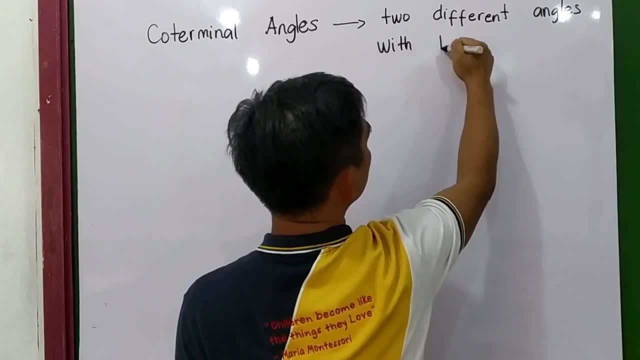 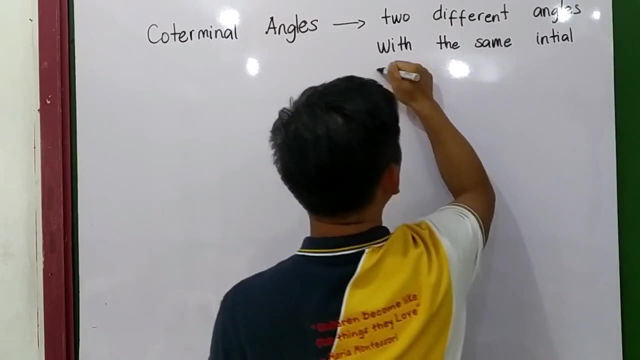 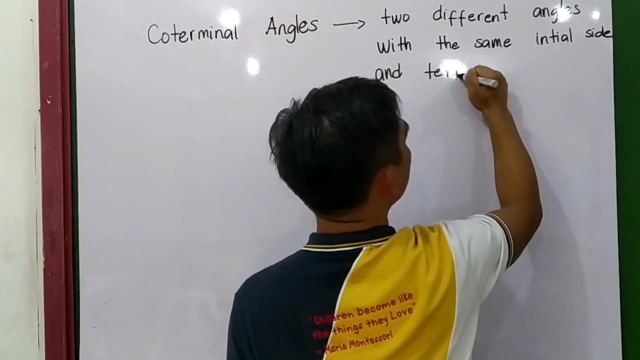 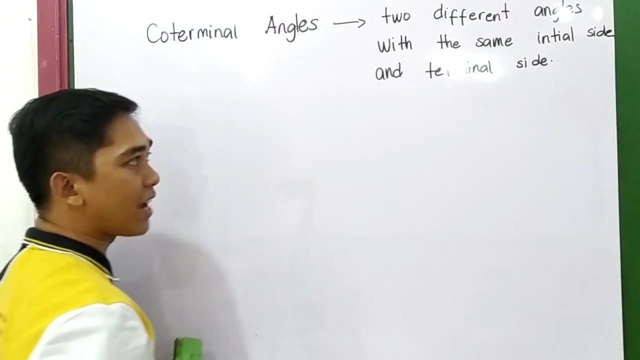 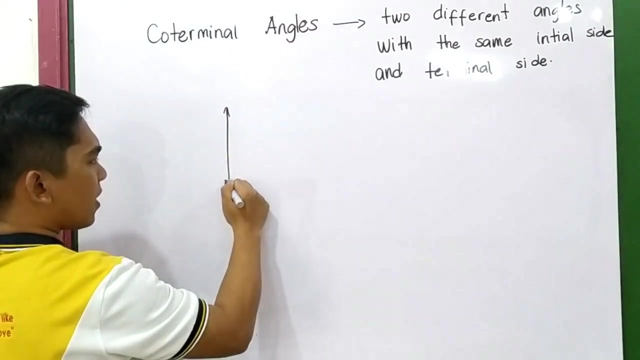 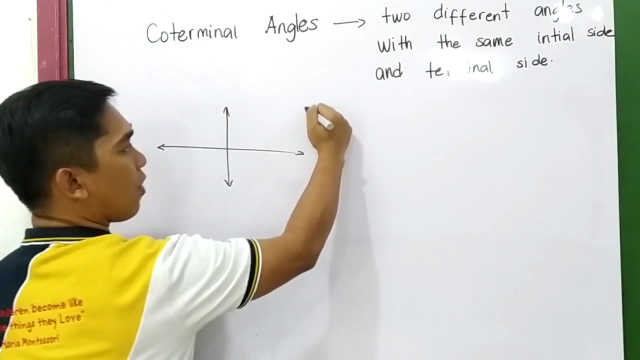 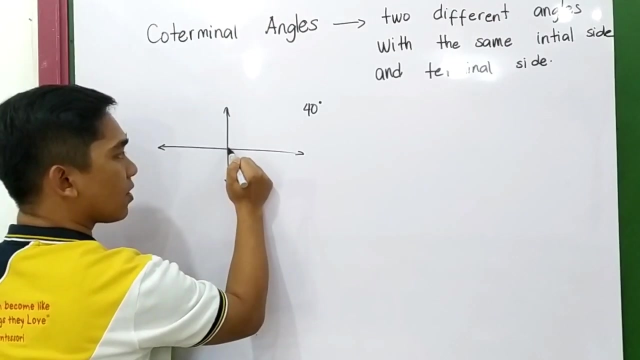 with the same initial side and terminal side. They have the same initial side and terminal side. Let us try to find the codeterminal angle of 40 degrees- 40 degrees, We know. 40 degrees is located between the first and the end. 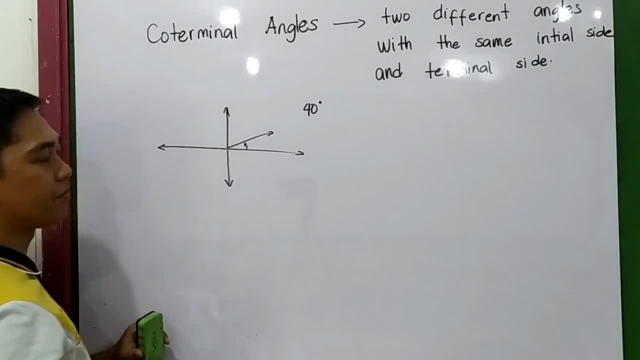 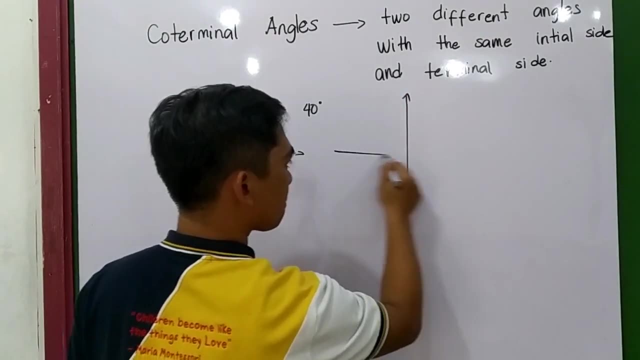 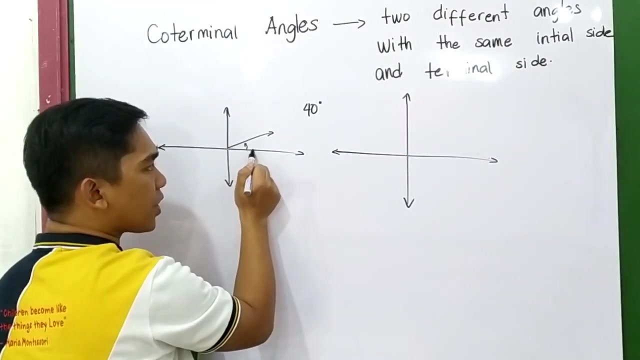 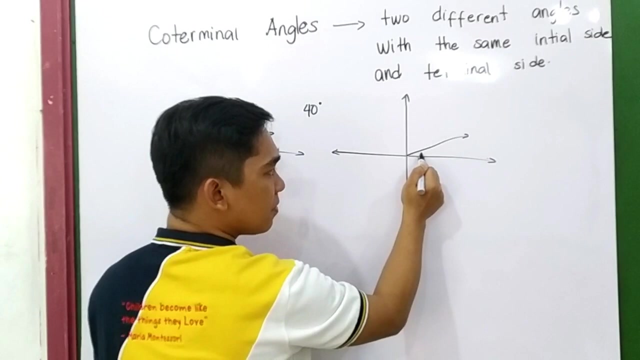 Here 40 degrees. Let us find the codeterminal of 40.. So our 40 is located here. So to find the codeterminal of 40, let us add 360.. So 40 is here. So 40.. 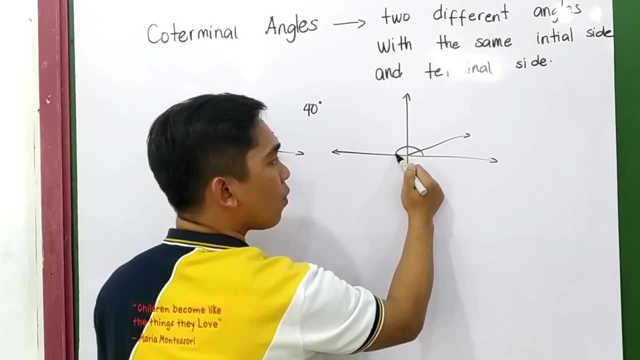 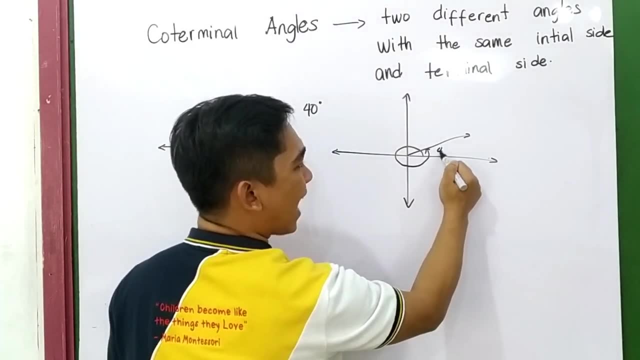 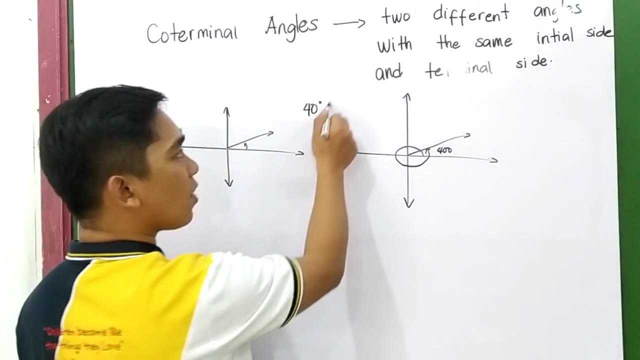 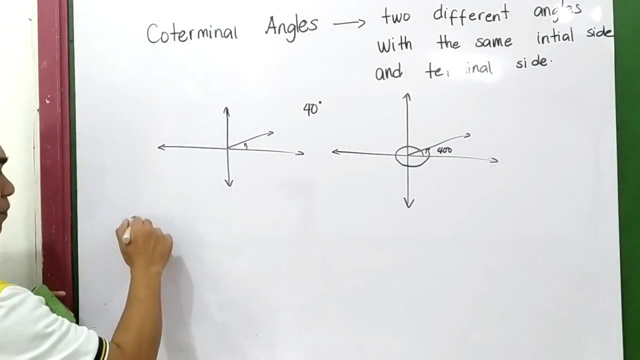 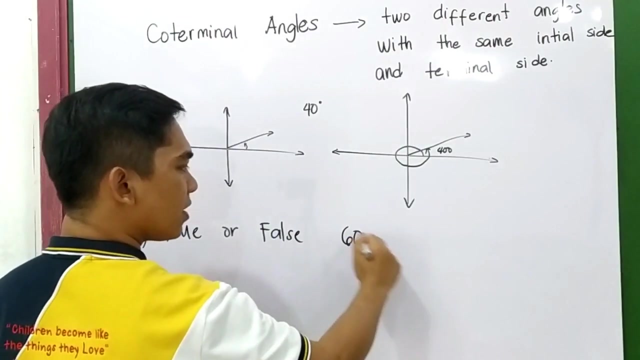 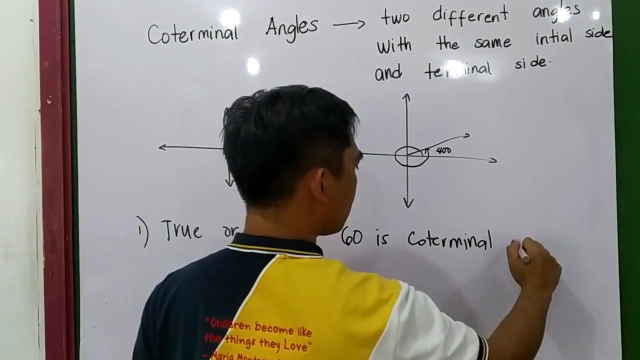 Then 90.. 180.. 270.. 360.. 360 plus 40. 400.. Therefore, the codeterminal of 40 is 400.. Let us try the question, true or false? 60 is codeterminal with 320 degrees. 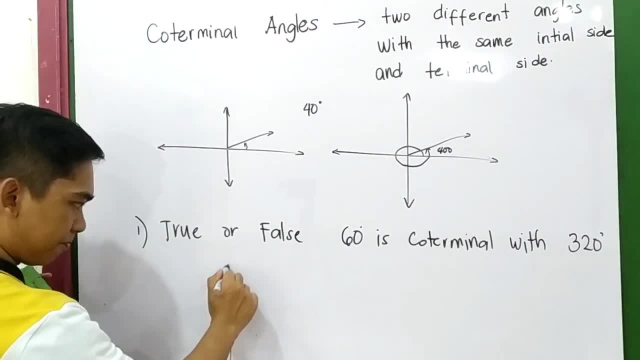 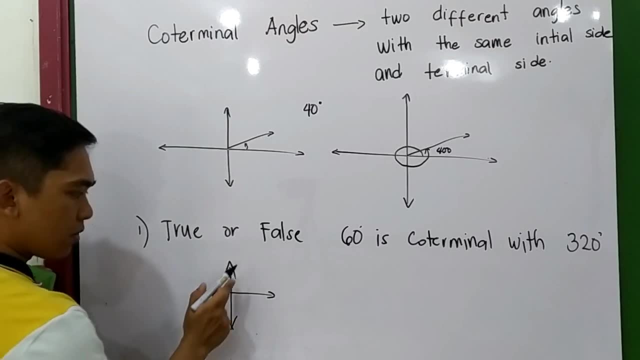 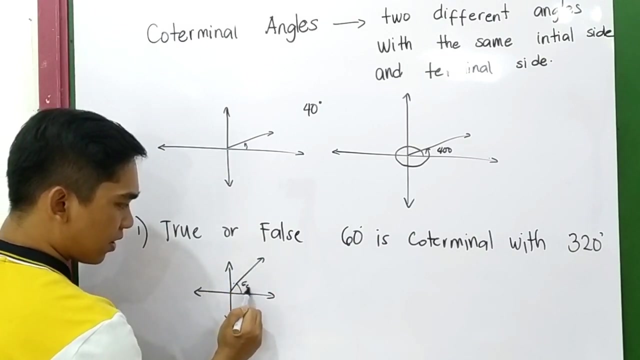 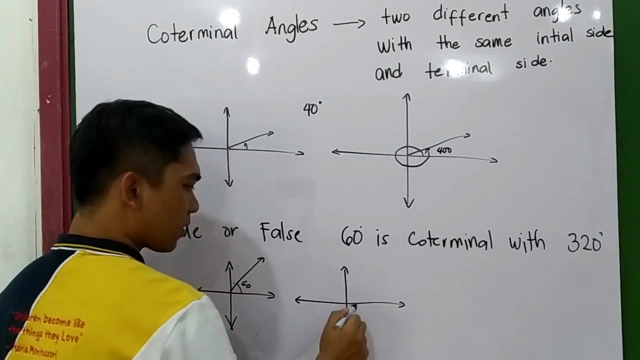 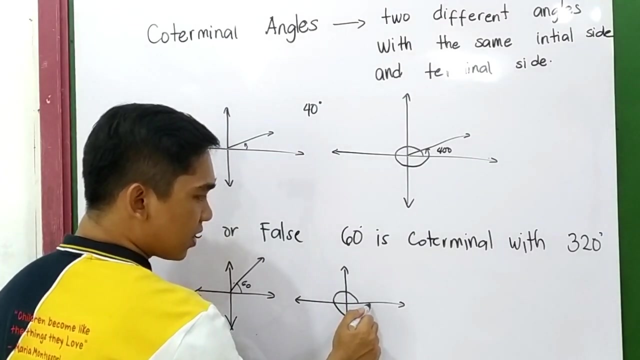 So let us find 60.. So 90.. So before 90 degrees, 60 degrees, Let us find 320.. 9,, 18,, 27,, 36.. 316.. So before 360 is 320.. Okay, 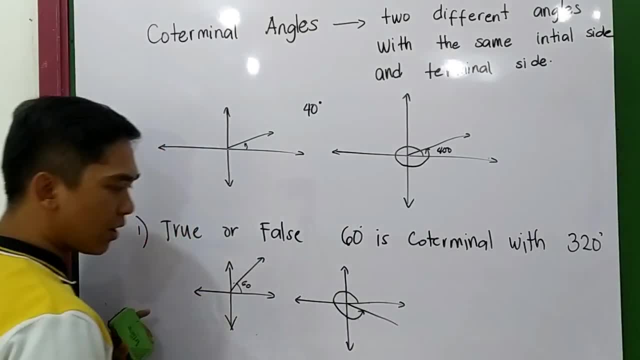 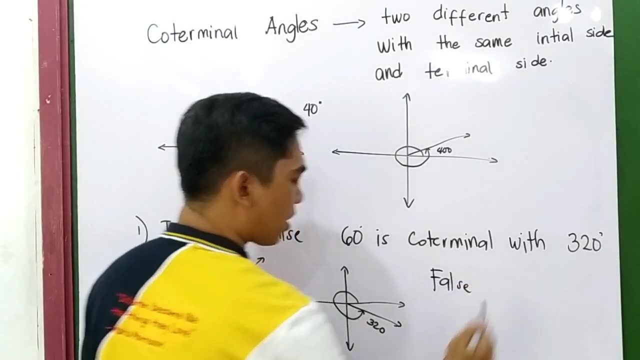 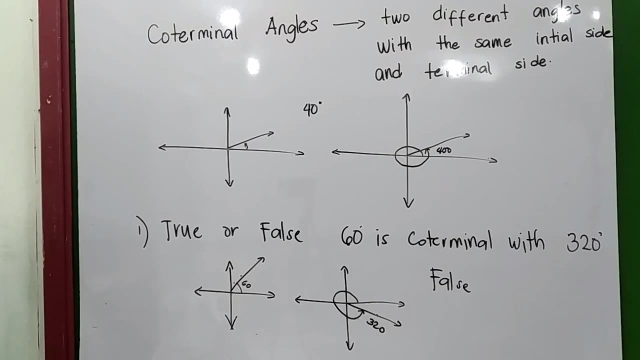 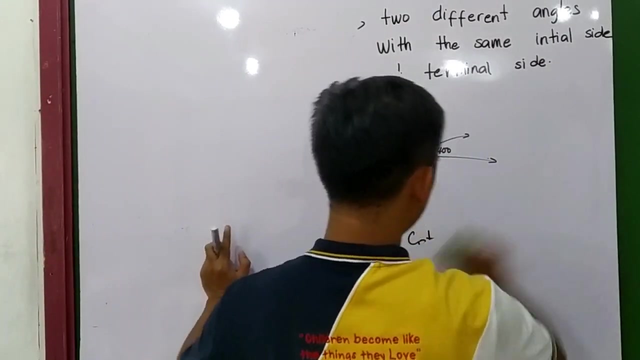 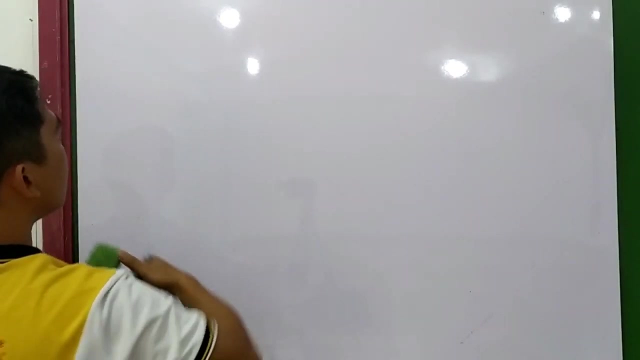 40 degrees. For false this is 320.. So other pseudonyms are false Because they don't have the same terminal time, Terminal space. Another definition is the contractile angles, Now, in this case the contractile angles up to the mental axis of the laughter. 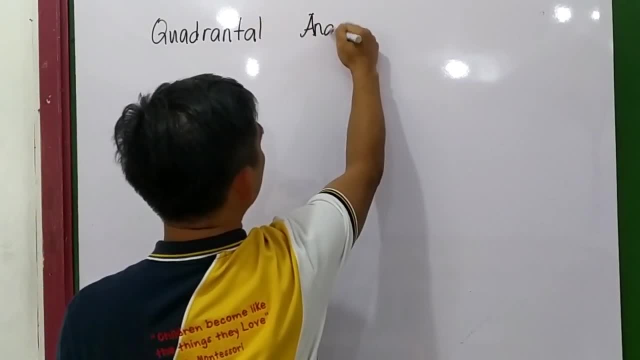 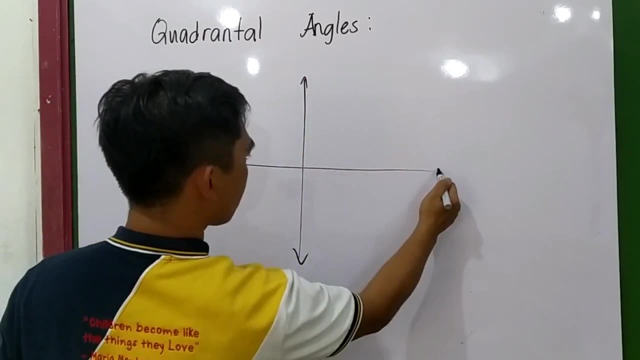 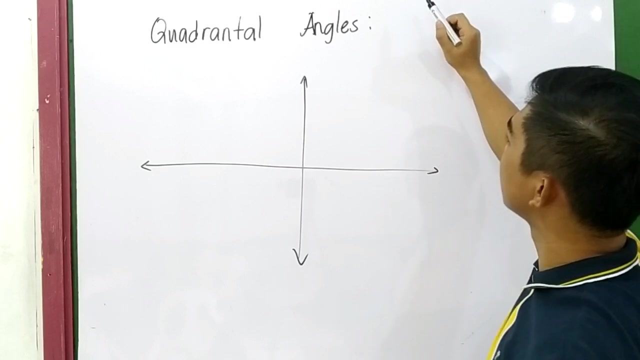 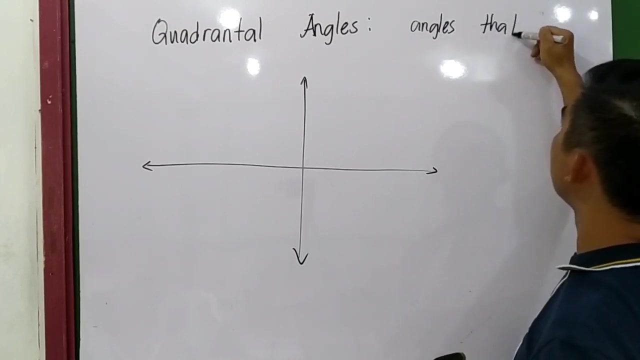 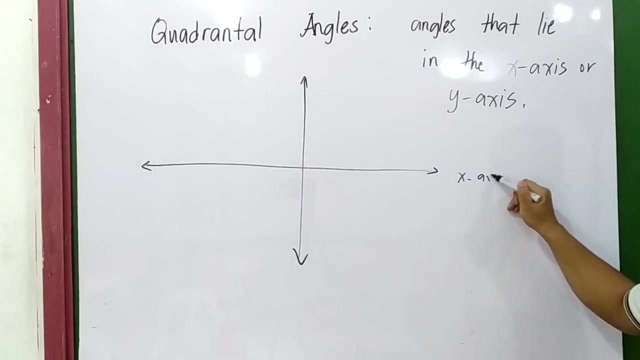 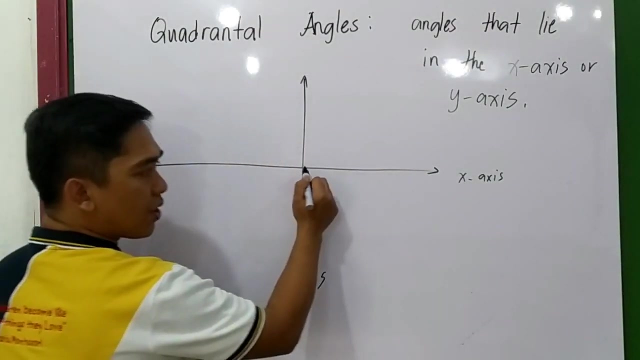 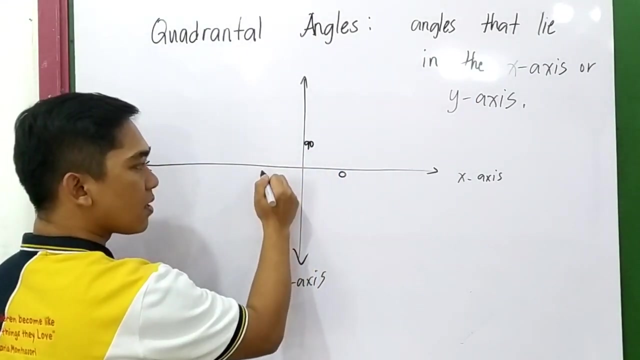 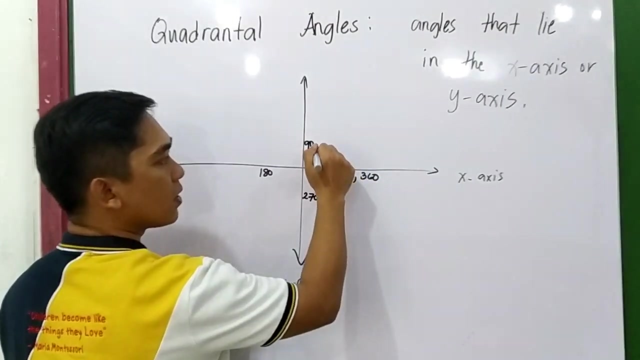 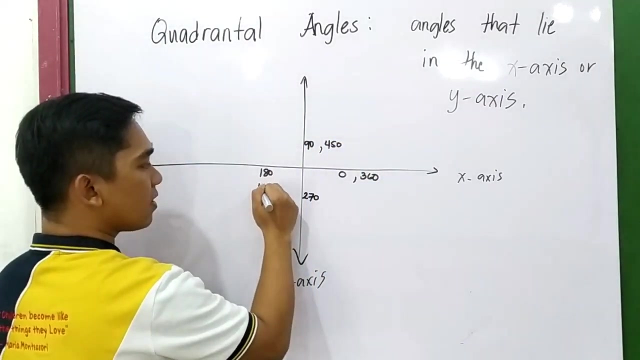 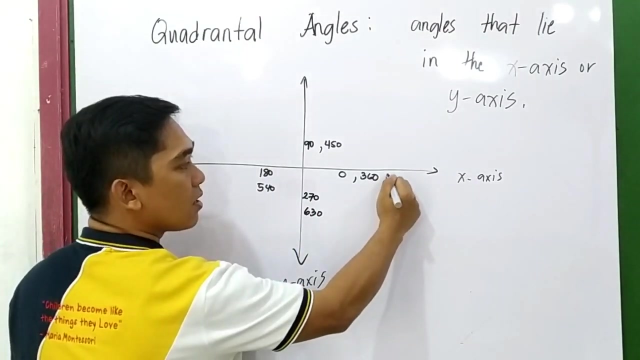 The contractile angles are angles that lie in the x-axis or y-axis, so this is the x-axis and y-axis, so zero lies in the x-axis, as well as 90,, 180,, 270, next 360, next 360, plus 90,, 450, 450 plus 90,, 540, 540 plus 90,, 630, 630 plus 90,, 720, 720 plus 90,. 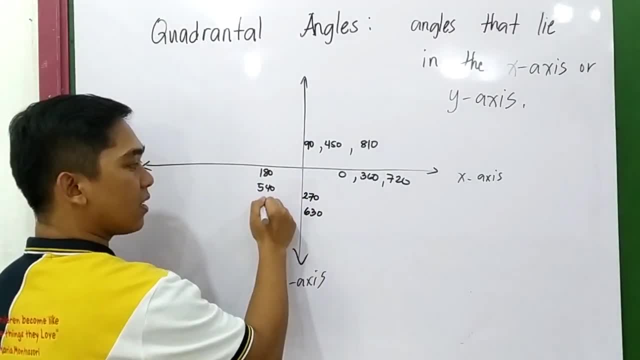 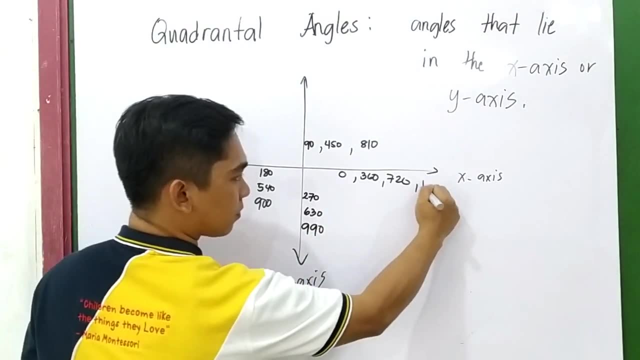 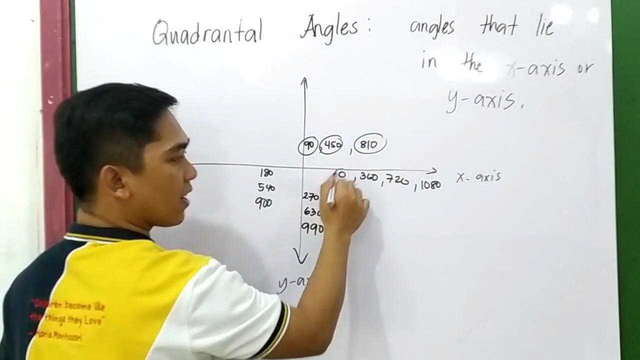 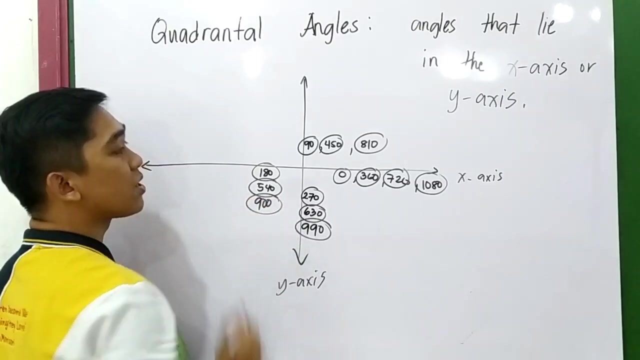 810, 810 plus 90, 900, 900 plus 90, 990, 990 plus 90, 1080, so these angles are our quadrangle angles, so you can memorize the multiples of 90,. those are the quadrangle angles. 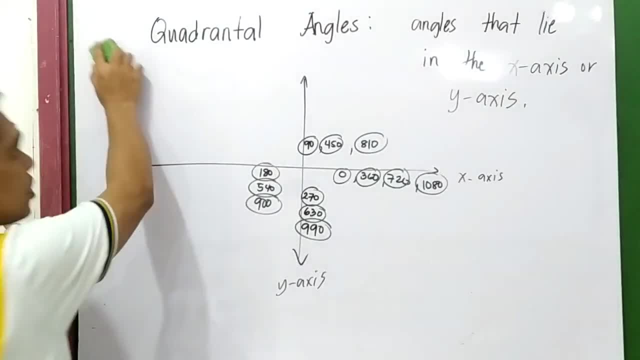 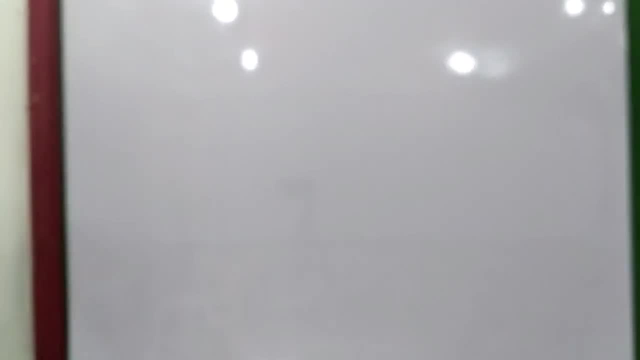 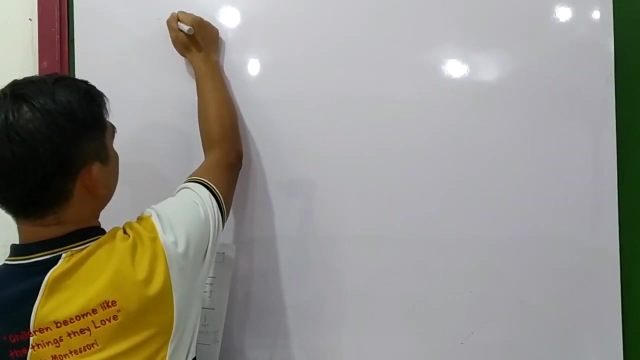 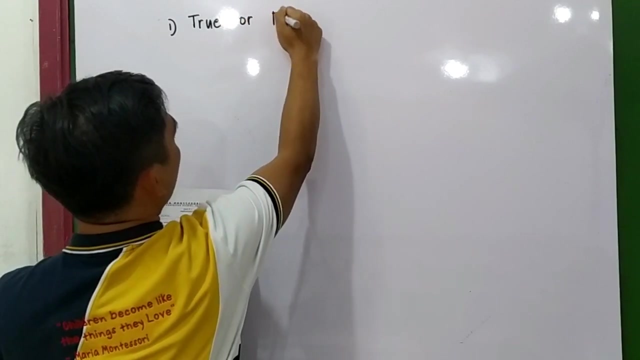 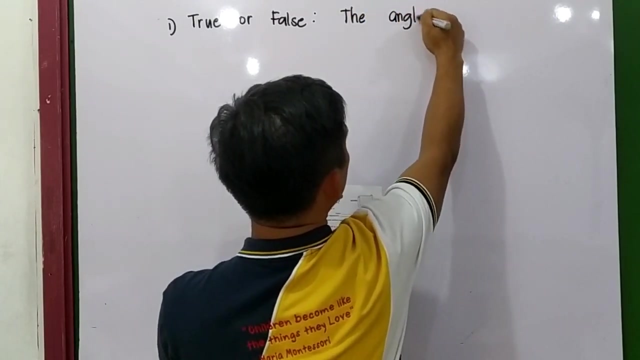 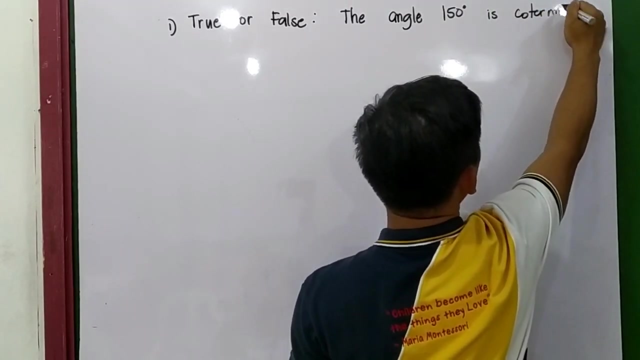 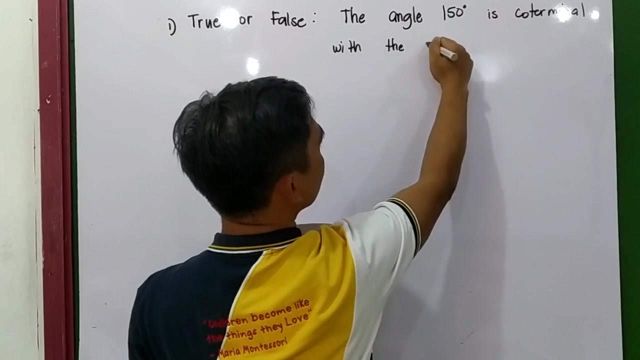 let us apply the differential equation. these are the 10 terms that we have discussed. ok, I have questions here. let us try 5 questions: true or false? true or false. the end: the outgel 150, 150 degrees is coterminal with the outgel 510 degrees. 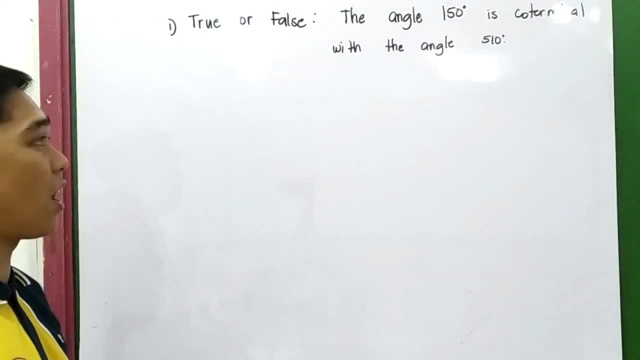 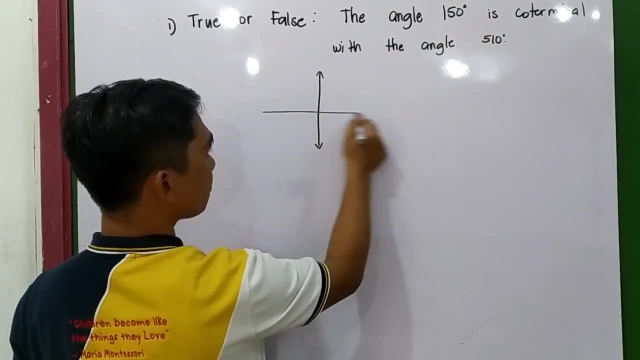 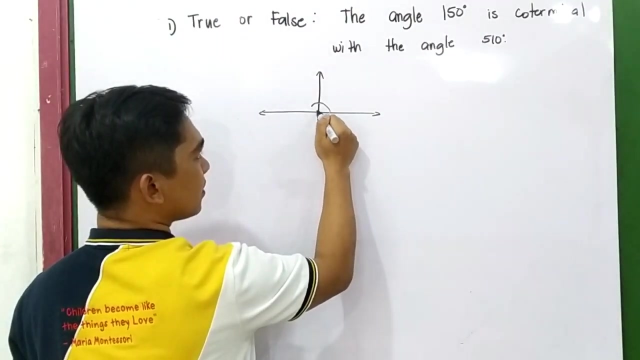 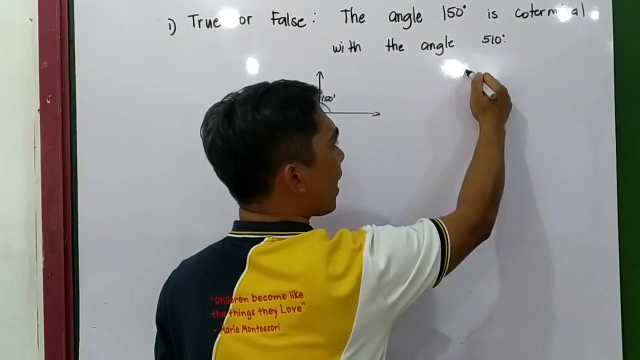 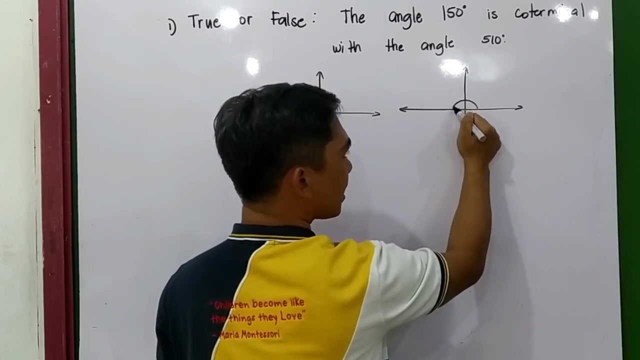 ok, let us check if they are coterminal. so 5150, 910, 90, so before 180, it is here. this is our outgel 150 degrees. let us find 510, 90,, 180,, 270, 360, one rotation. 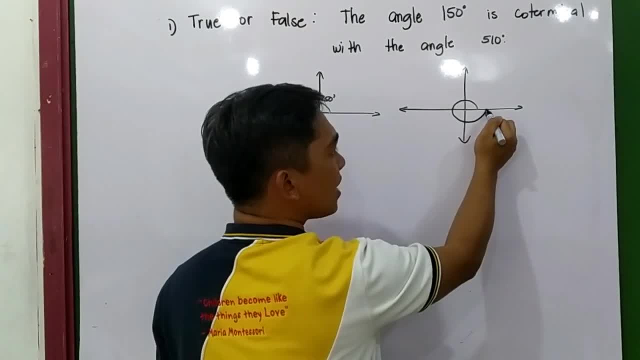 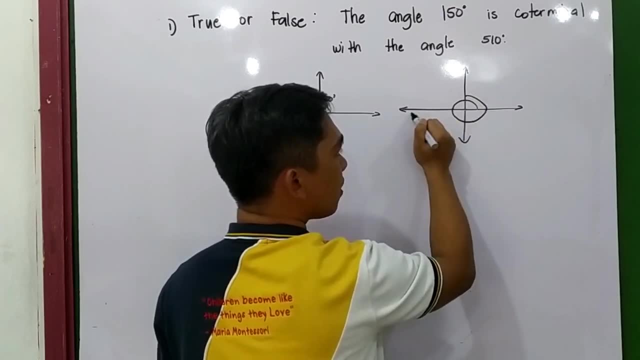 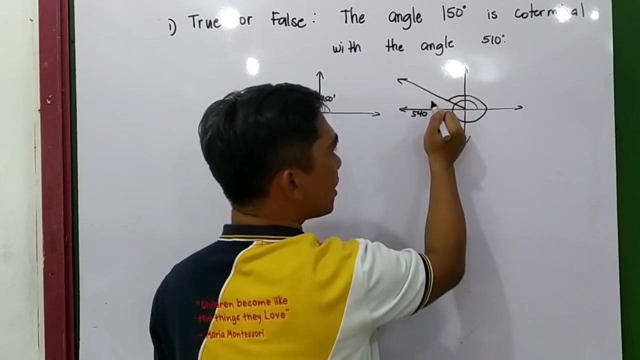 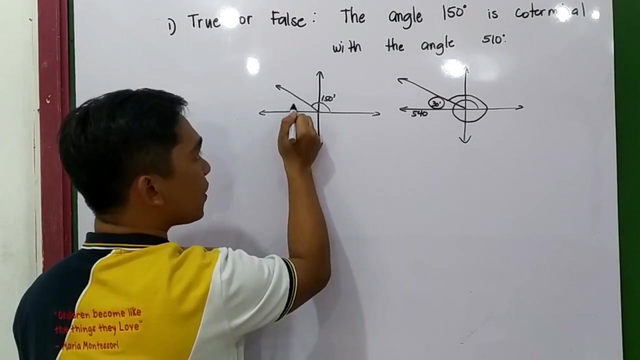 360 plus 90,, 450,, 510,. Next is 450, before 450,, so it is 540.. So before 540, 510.. 30 degrees before 540.. How about here? 30 degrees before 180.. 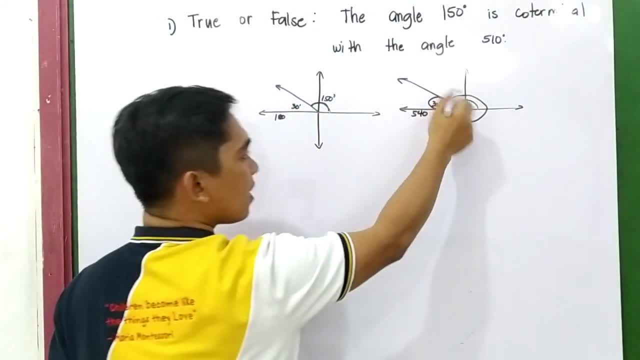 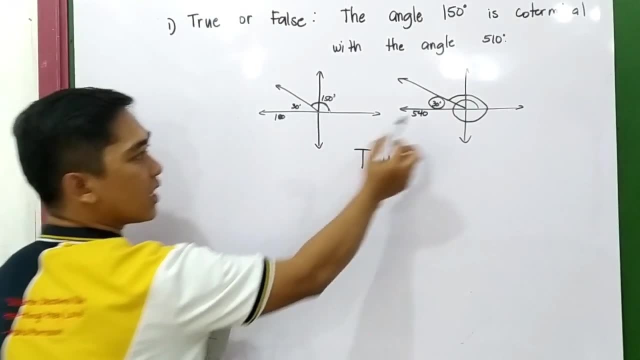 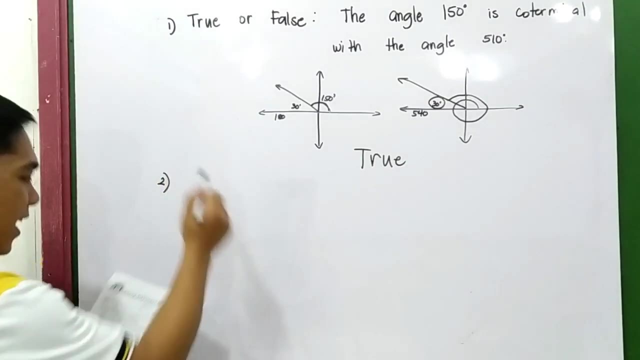 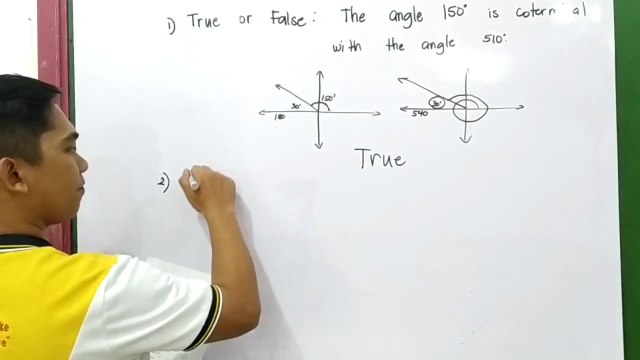 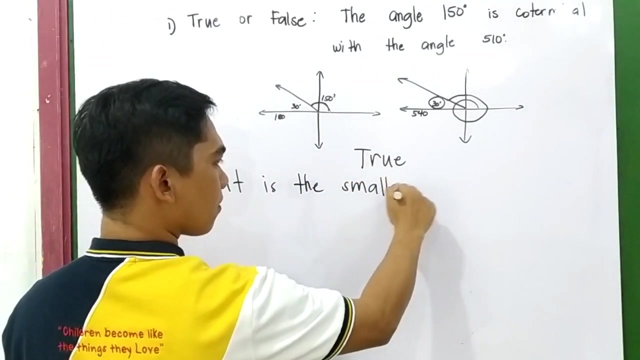 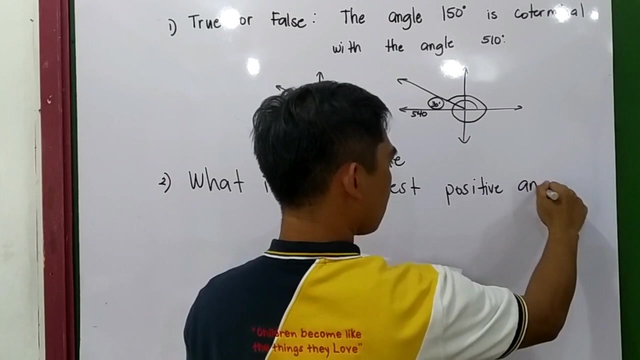 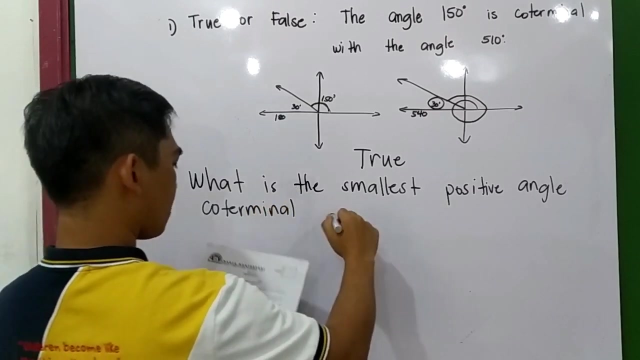 That means the two angles are coterminal: 30 degrees before 180,, 30 degrees before 540, they have the same terminal size. Second example: What is the smallest casting angle coterminal with negative 45? Negative 45.. 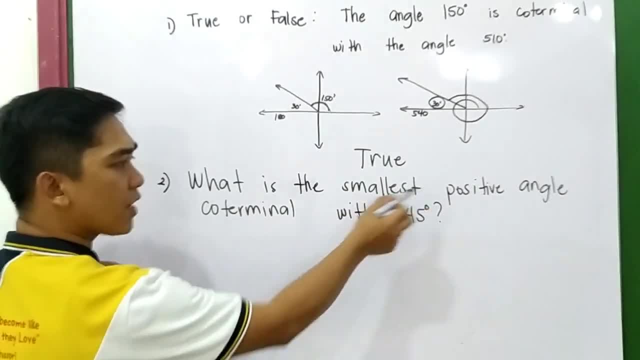 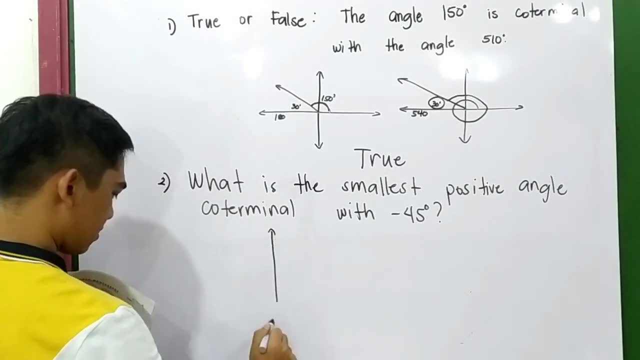 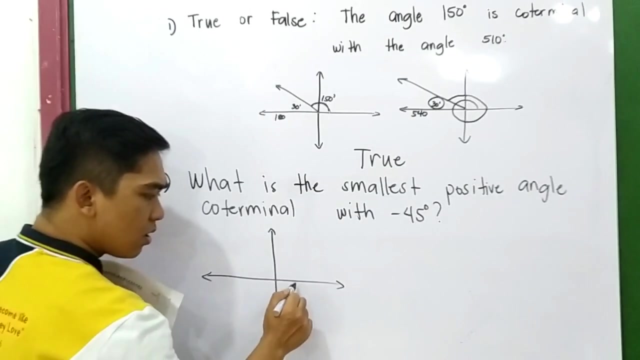 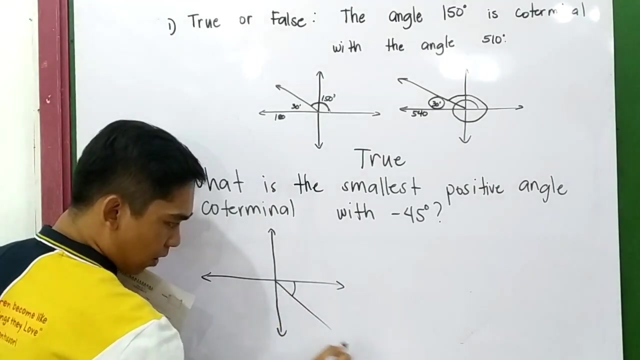 Ok, Negative, or smallest casting angle coterminal with negative 45. Let us find out for this negative 45.. Let us find out for this negative 45. Let us find out for this negative 45.. Negative 45, Negative. so the angle rotates clockwise direction. 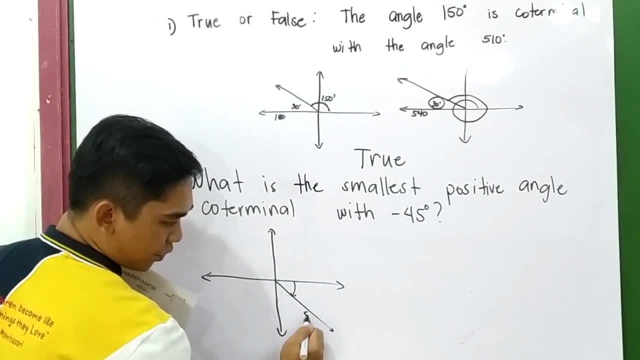 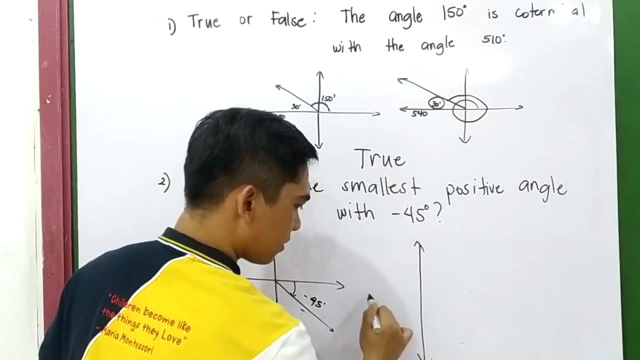 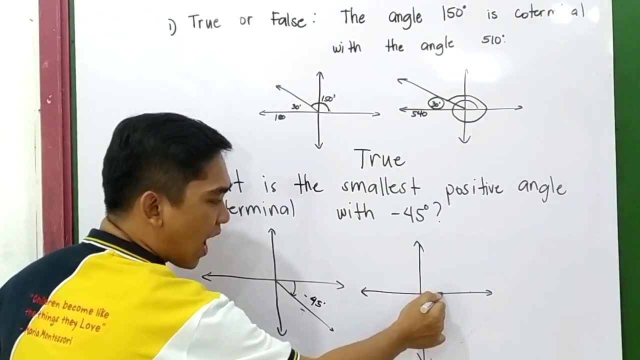 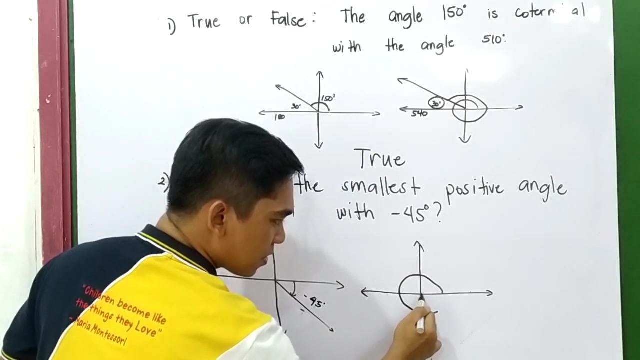 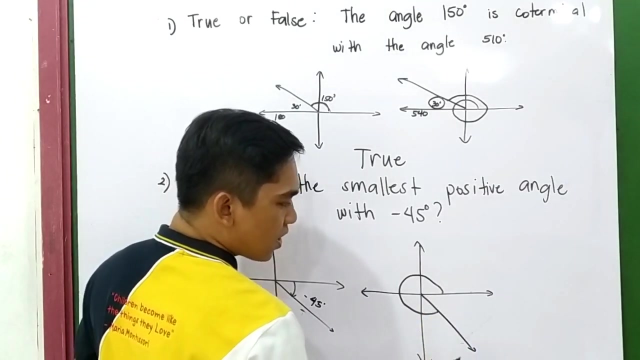 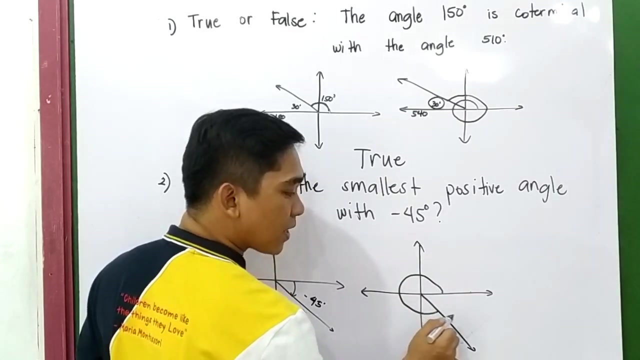 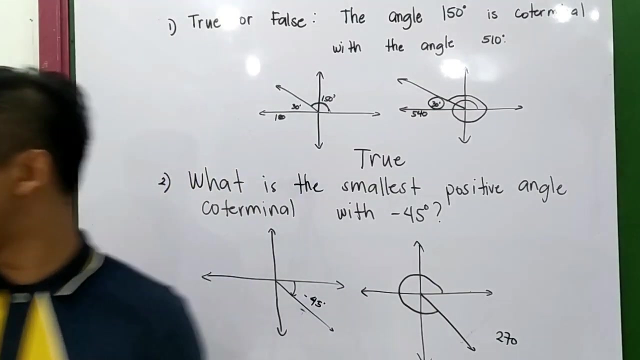 45 degrees Negative, 45 degrees Positive. So from our initial sign, rotate counterclockwise, It's positive. It's between 4 quadrants, So 90, 180, 270, So 270, plus 45, So 270. Let us add 270 to 45. 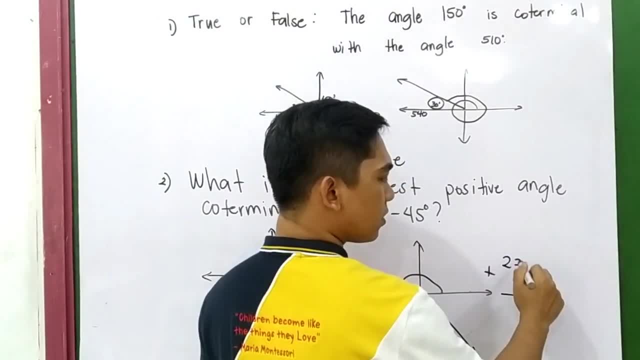 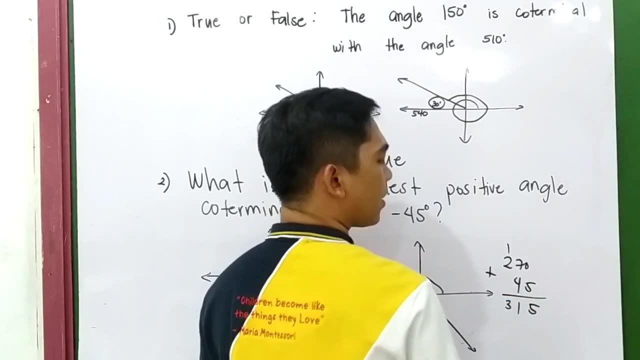 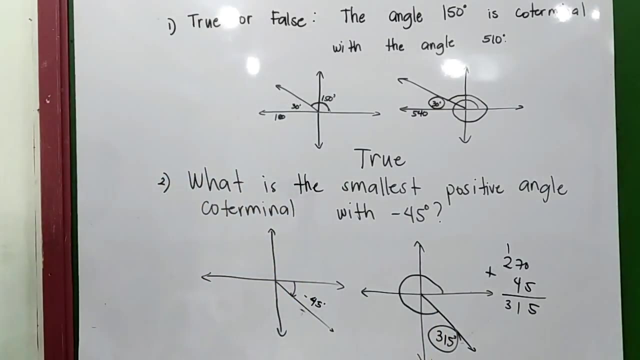 270 plus 45, 0, Sorry, 0 plus 5, 5, 11 care 1, 300 degrees. Therefore, this angle is 300 degrees, Which is Co-coordinal, The smallest co-coordinal of negative 45 degrees. Third example: 0 is 30 degrees. 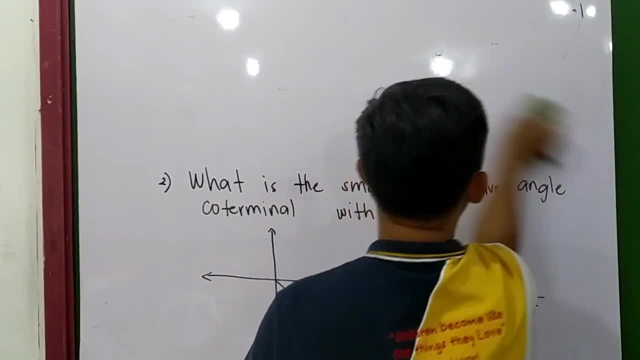 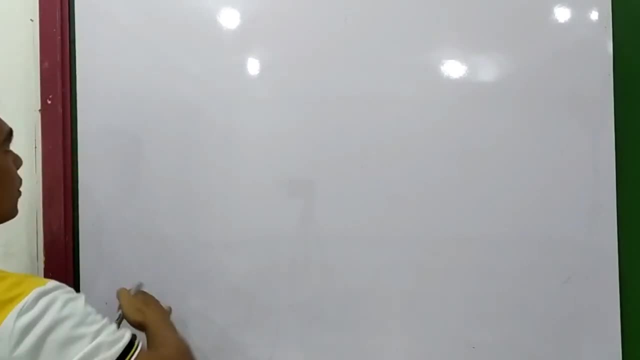 So if 4 is straight, then it is 90 degrees, So the angle is 20 degrees, And left side of the curve is 1 degree, So 2 degrees. So the angle of the curve is 20 degrees, Which is 12 degrees, So the angle of the curve is 10 degrees. 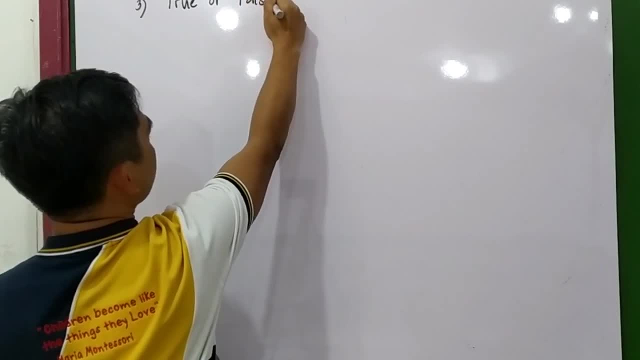 So if 3 is straight, then it's 90 degrees. The angle of the curve is 7 degrees. So if 4 is straight, then it is 74 degrees, But in this example it's 20 degrees. It means that I'm not going to turn it over. 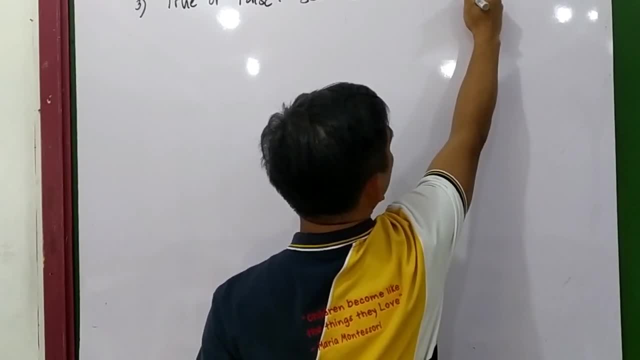 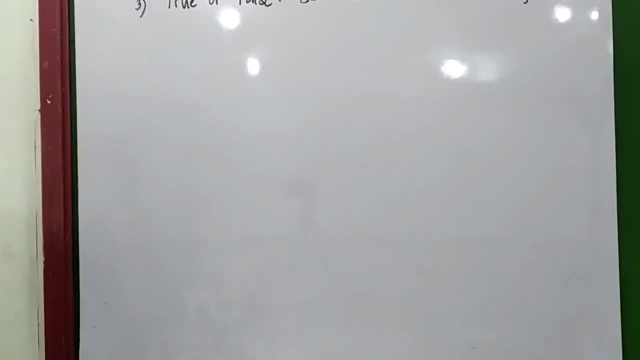 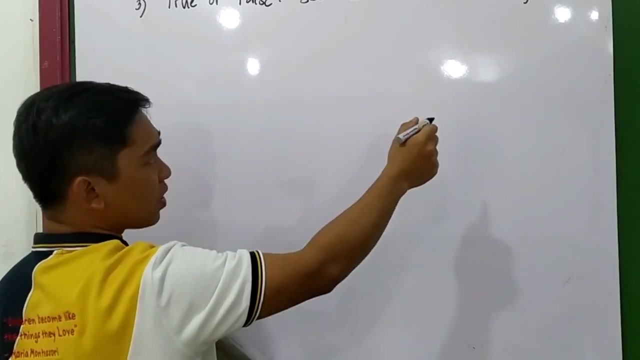 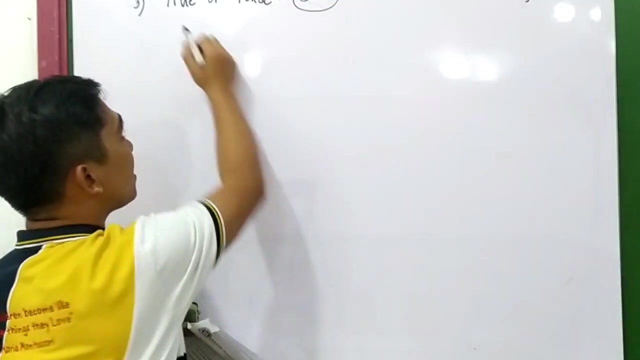 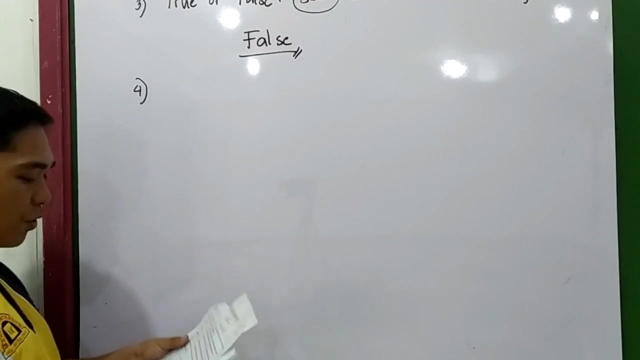 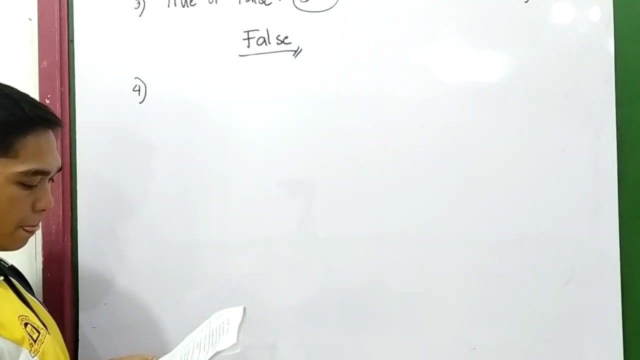 So we have to make a few changes. angle. So where is 820?? So we know that quadratal angles are multiples of 19.. Is 820 multiple like 19?? No, So that means this is same, as it's almost Number four. Number four, the. 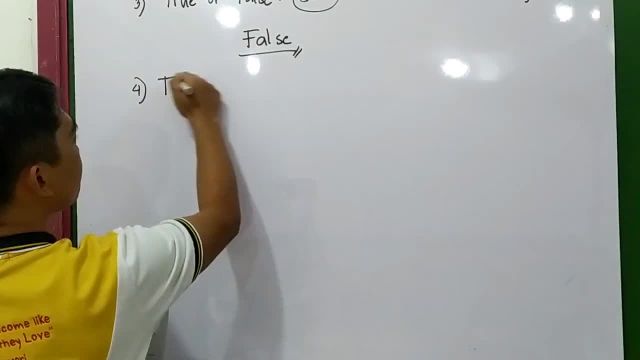 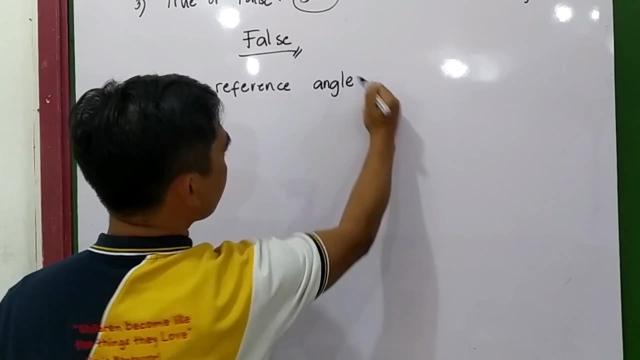 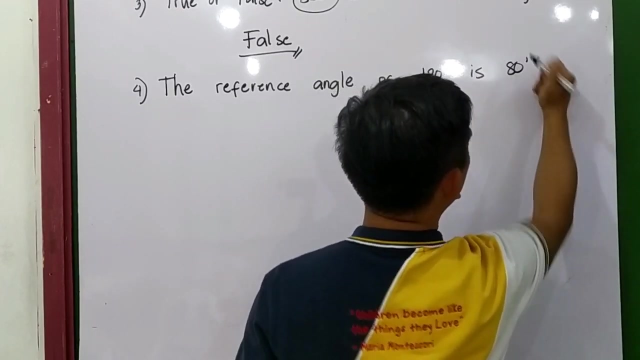 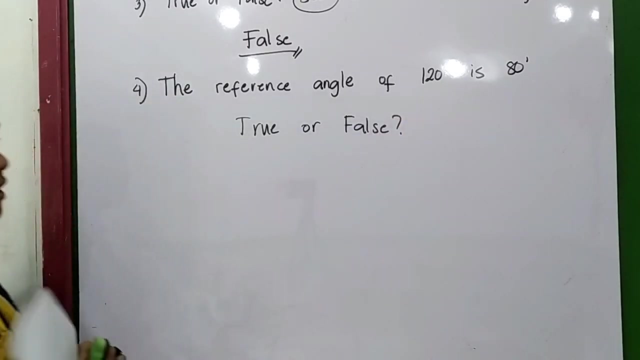 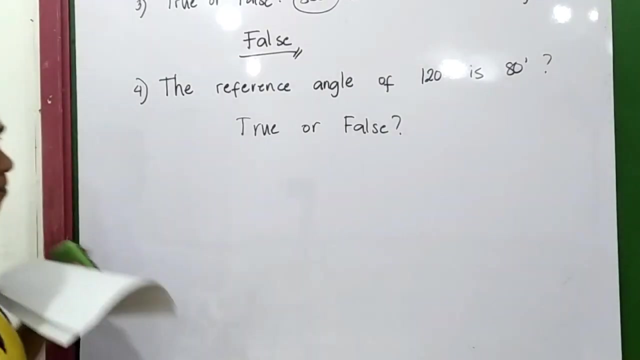 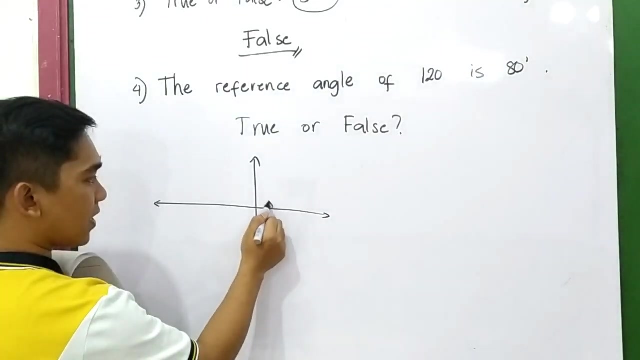 reference angle of 120 degrees. Reference angle of 120 is 80 degrees through our holes. Reference angle of 120 is 80 degrees to our holes. So let's check: Where is 120?? So 90 plus 30, 120.. So this is 30.. Before we reach 80,, we need 60 more. 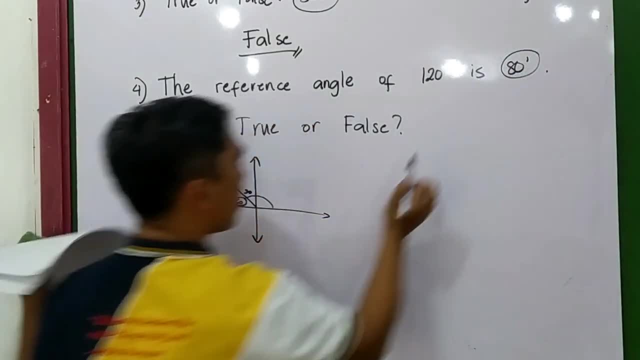 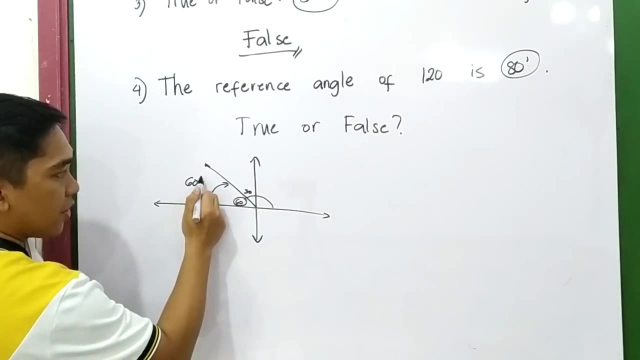 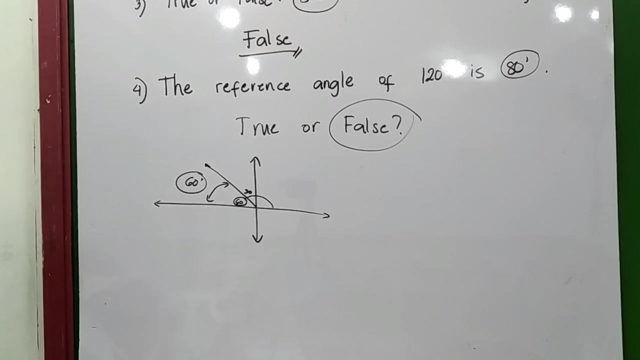 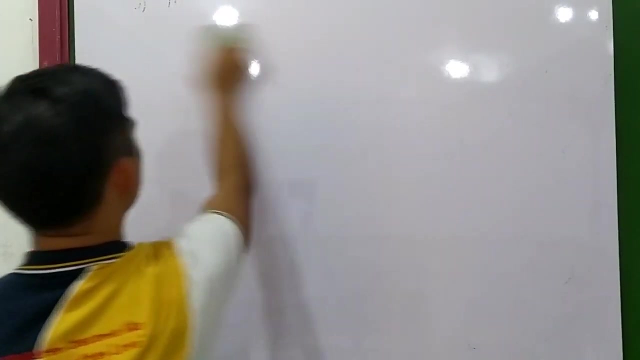 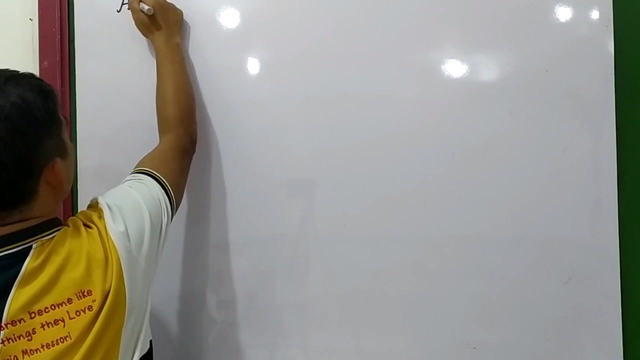 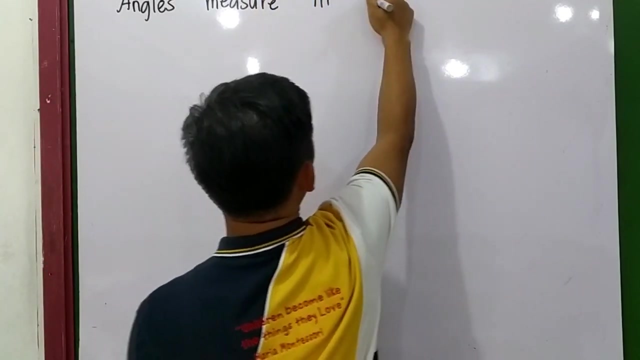 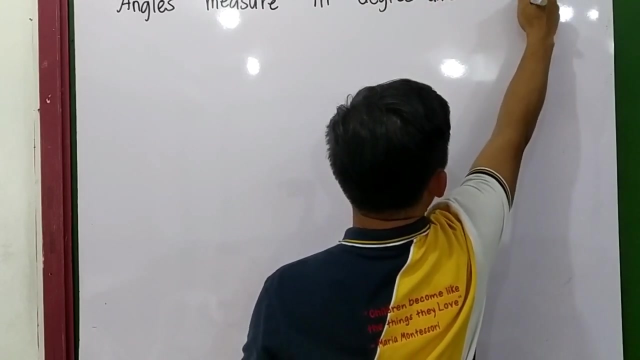 So 80 is not the reference point, because our reference angle is this angle measures 60. So the answer is 60.. Next, Our next lesson: Angle measures in degree and ratio. Angles measure in degree and ratio. So 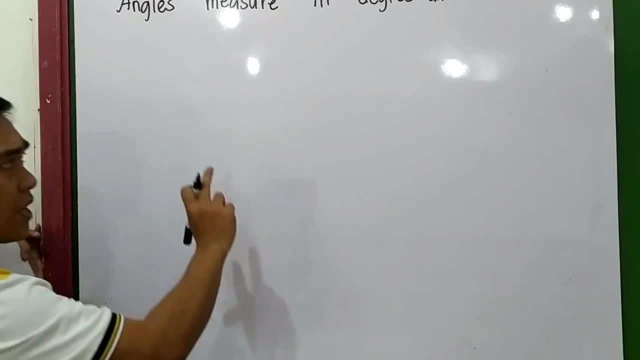 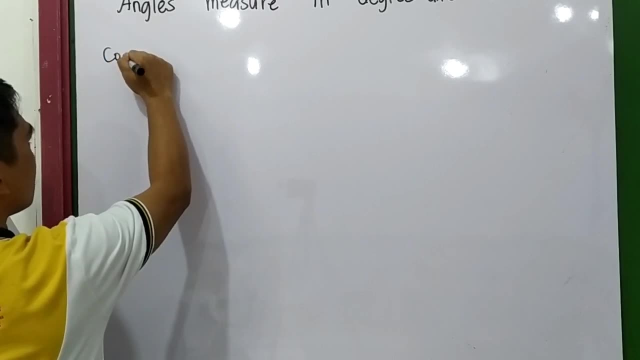 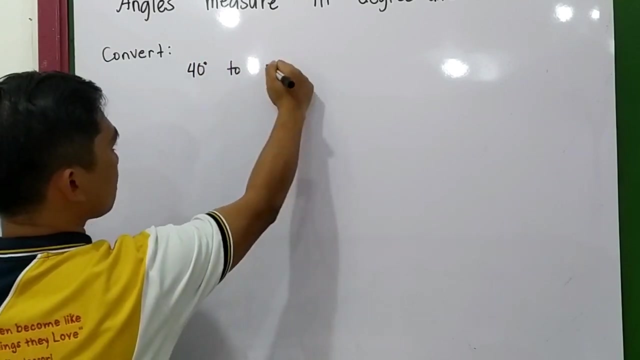 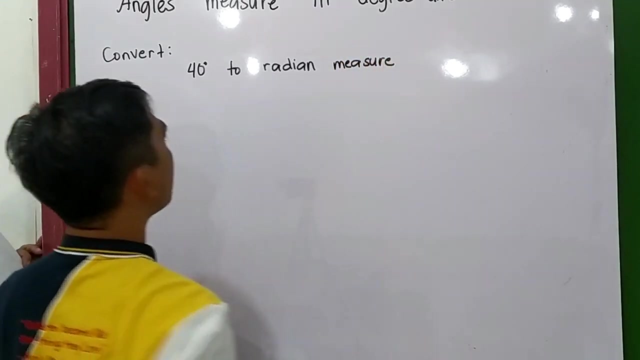 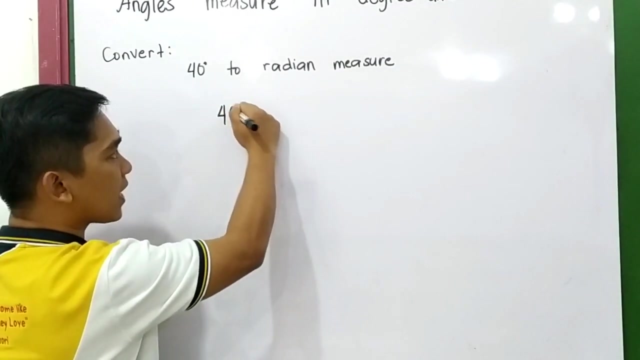 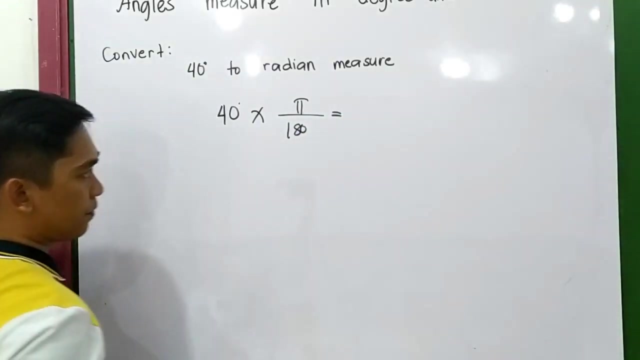 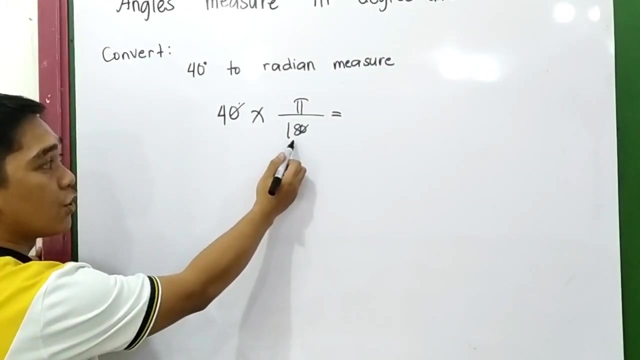 We need to convert from degree measure to ratio measure. Let's say we have Convert 40 degrees angle to ratio measure. So in order for us to convert, multiply the given angle to pi over 180.. So cancel 0.. 4 and 18 are divisible by 2.. 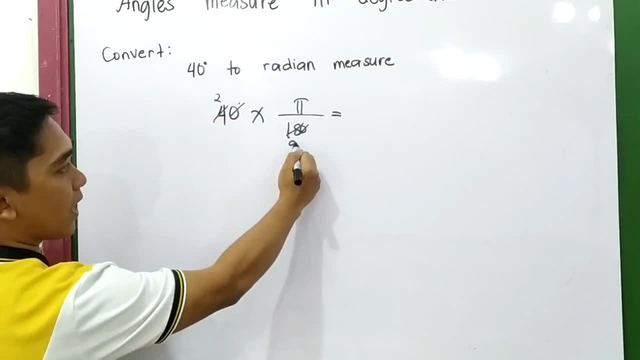 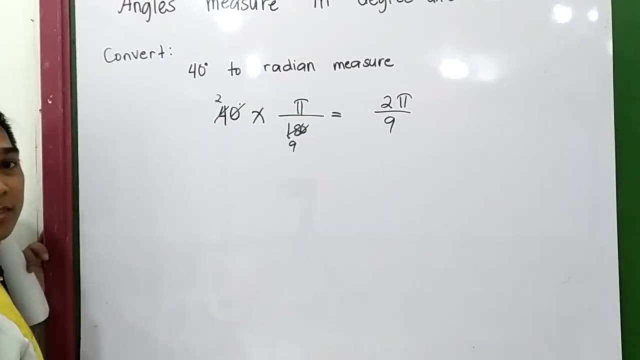 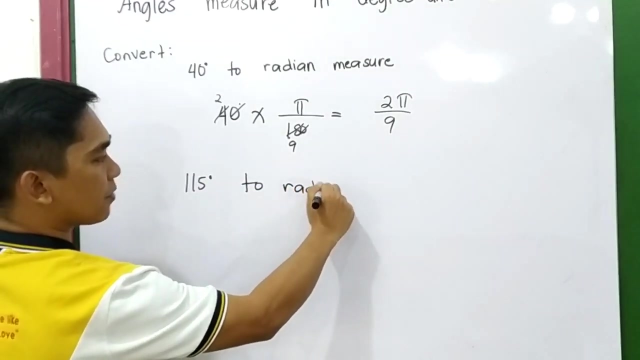 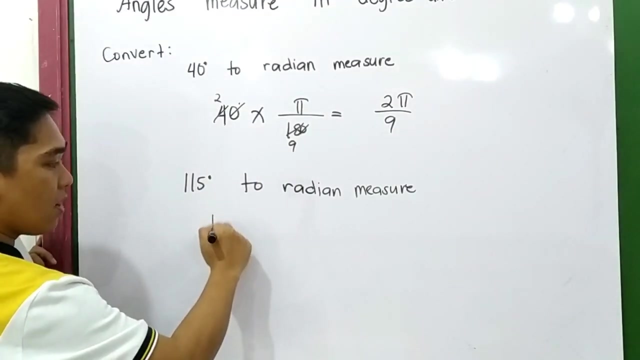 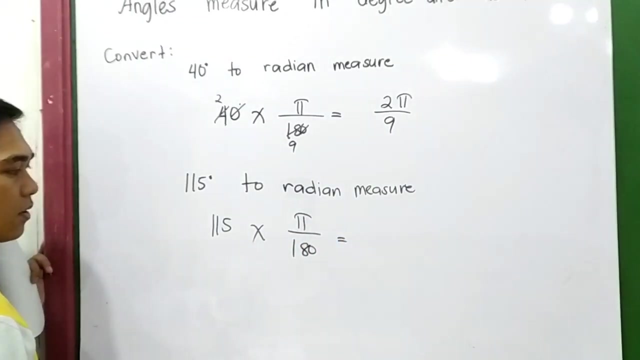 So cancel 4.. 2,, 18,, 29.. So the ratio measure is 2pi over 90.. Next Convert 150 degrees to ratio measure. The same formula: 115 times pi over 180.. So 115 and 118.. 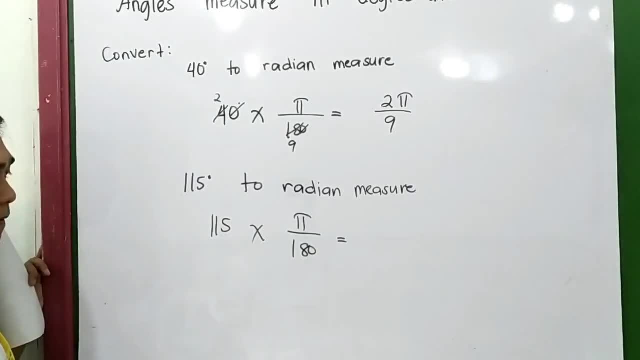 They are divisible by 118 And 126.. Are they divisible by 3? 115 divided by 3.. 1, 9.. 2, 9.. 1, 9.. 3, 9.. 2, 9.. 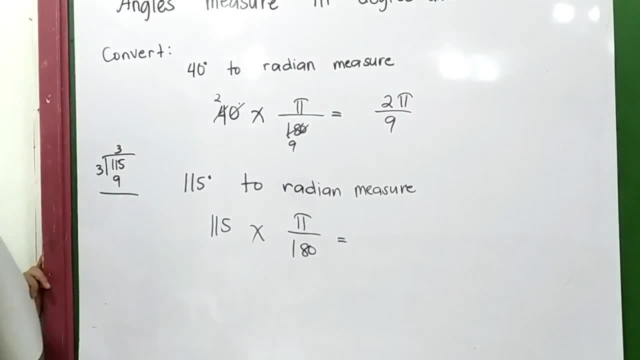 1, 9.. 1, 9.. No, they are not divisible by 3.. They are not divisible by 2.. The first is 1, 9.. 1, 9.. The second is 1, 9.. 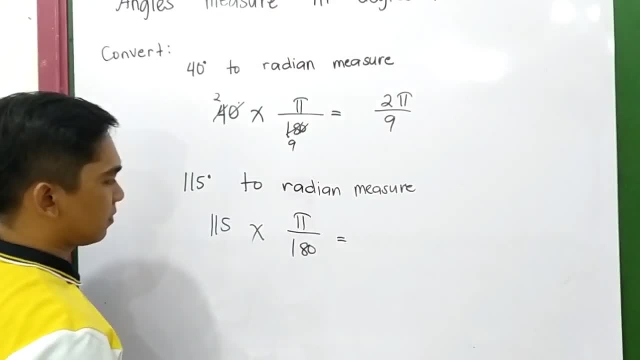 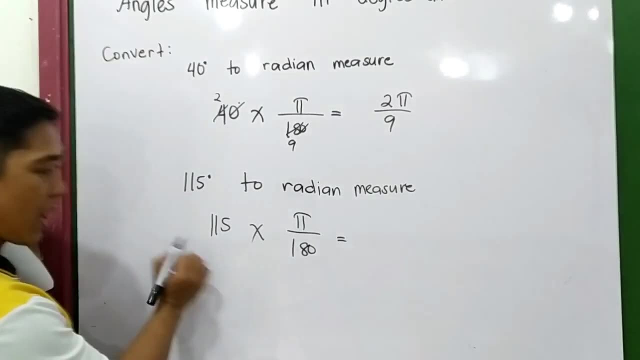 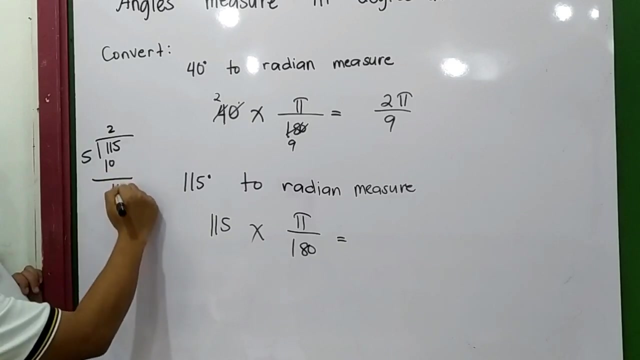 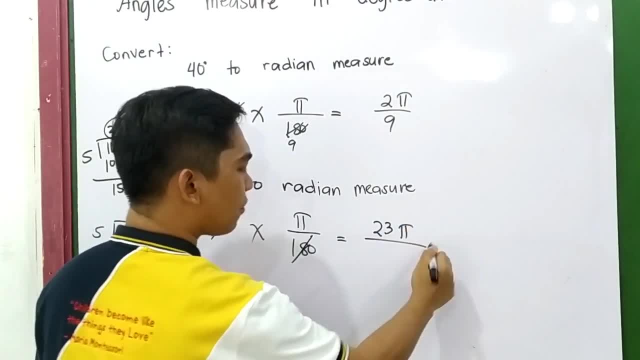 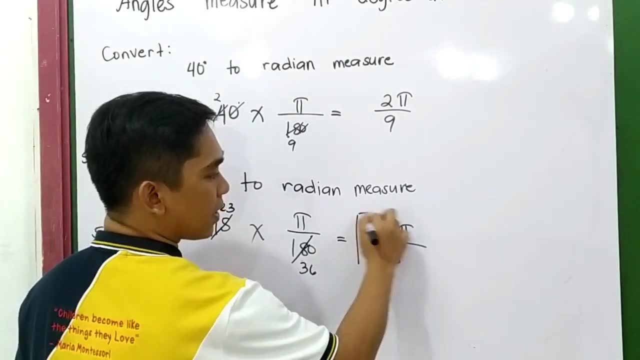 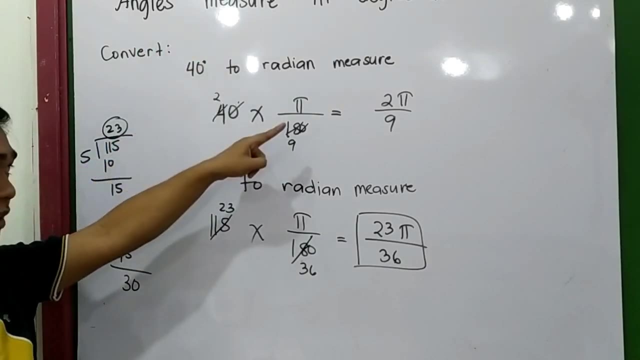 So we have 23 pi over 180 divided by 5, this is 36,, so 36 in the denominator. Now the formula. The formula is the given sample converted to range of pressure is multiplied to pi over 180.. What is the given is range of pressure converted to degree of pressure. 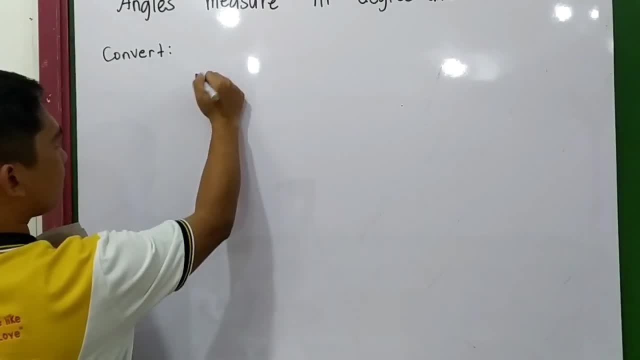 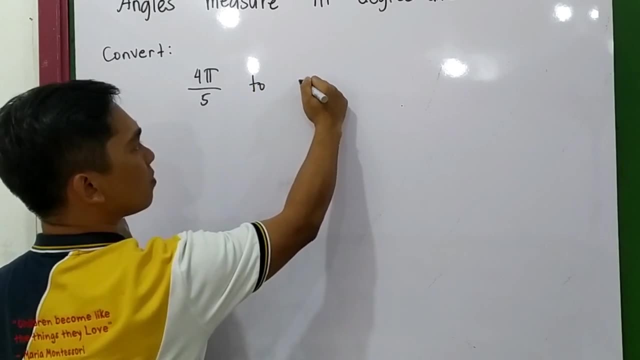 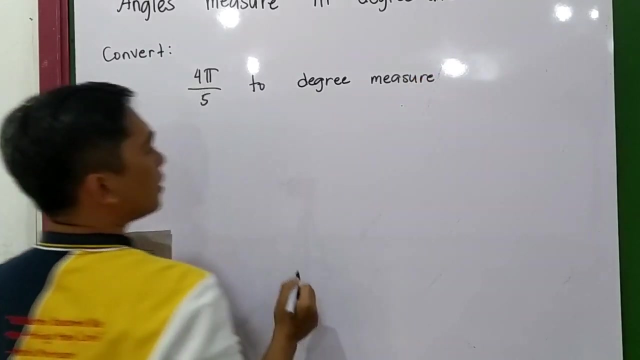 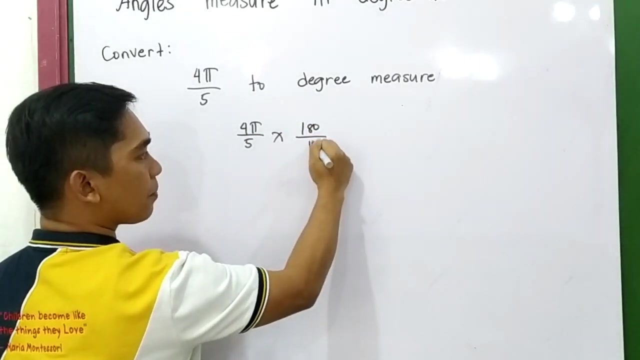 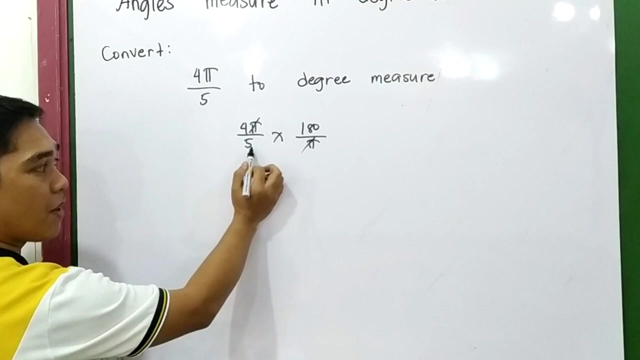 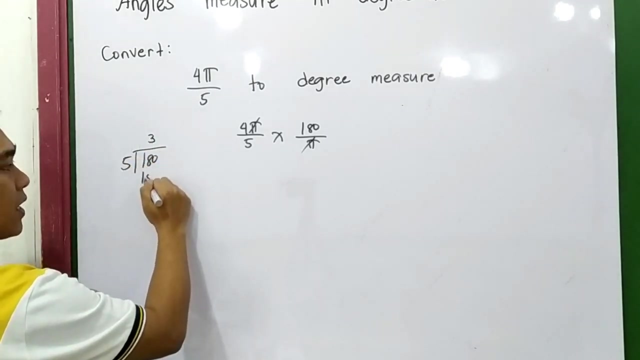 Let's try 4 pi over 5.. Convert 4 pi over 5 to degree. Measure 4 pi over 5 times 180 over pi. So pi 180 divided by 5, 180 divided by 5, 3 times 3,, 15,, 30.. 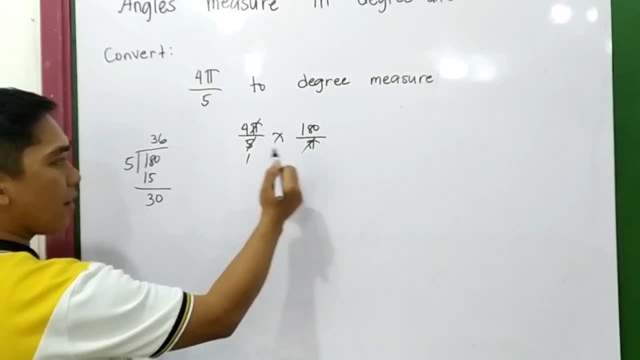 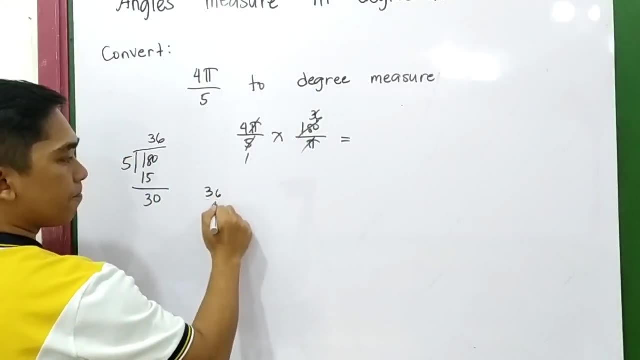 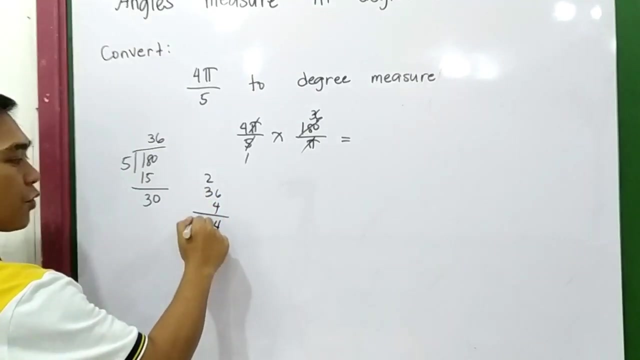 36. 36. And so pi changed to 36. Now, 36 times 4 is 6 x 18,, 24,, 32, or 34,, 144.. 144.. Yes. Second example: 7 pi over 5.. 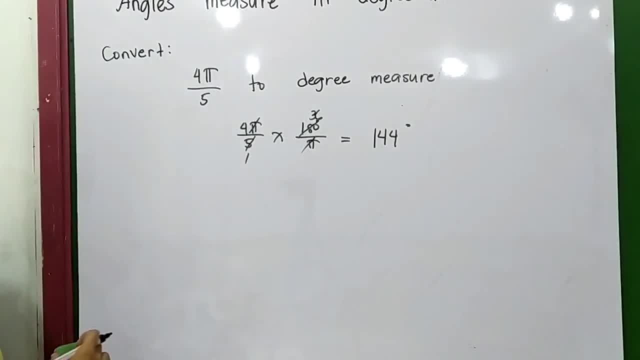 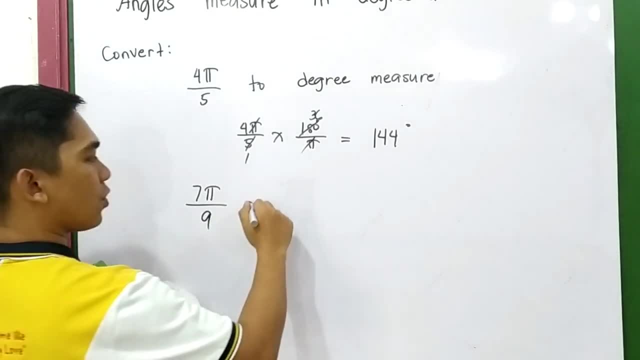 7 pi over 9.. 7 pi over 9.. 2 degree measure. So 7 pi over 9 times 180 over pi, osing number 9.. 7 pi over 9 times 180 over pi. Cancel pi. 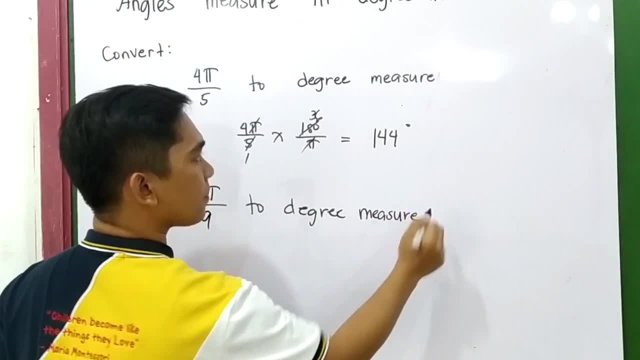 180 is possible times 9.. So cancel that 20.. Okay, 7 pi So 7 times 20 is equal to 100.. 120 means to hear the right answer, N, So 8x50 equals 100.. 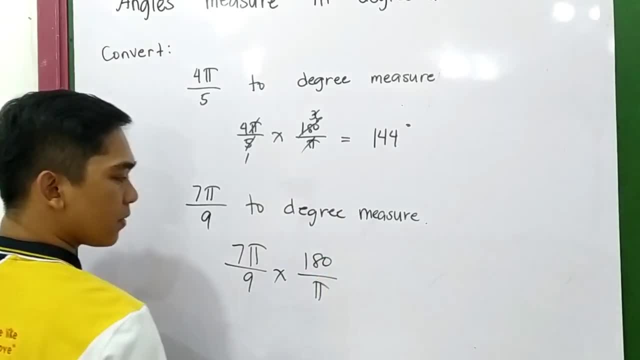 7xcity equals 10, so 3xc Greadows is equal to 1 every time, What does this key terms equal to? When the caseley changes, all the values on this system are the actives and the後. 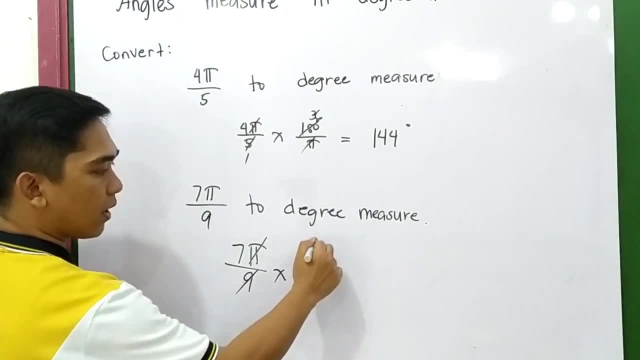 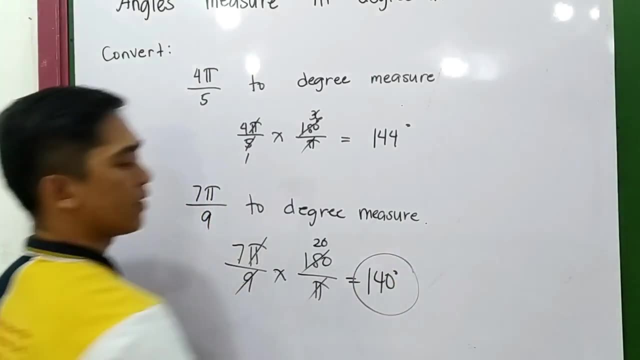 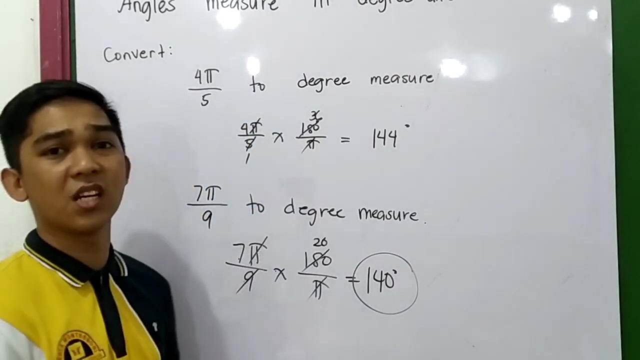 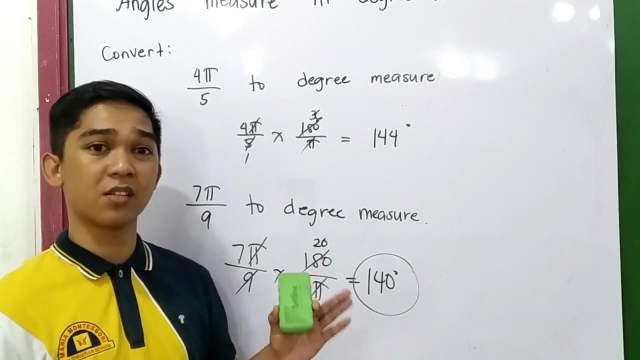 or non. So output P must have a value. New change compared to This is A logic Correction. clients It. Okay, Let us summarize our lesson. So we have the angles in the coordinate plane If our vertex is located in the origin. therefore, that is in the standard form. 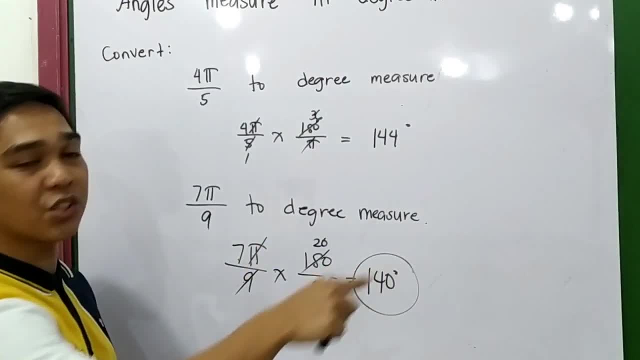 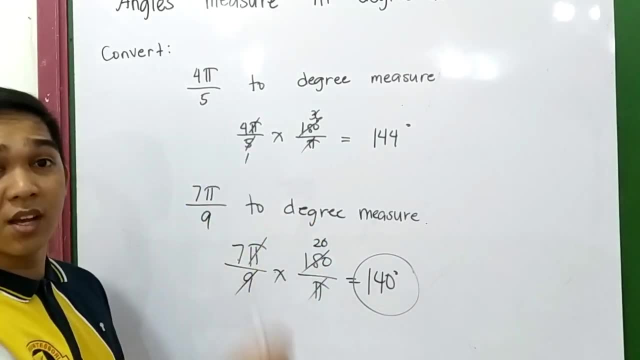 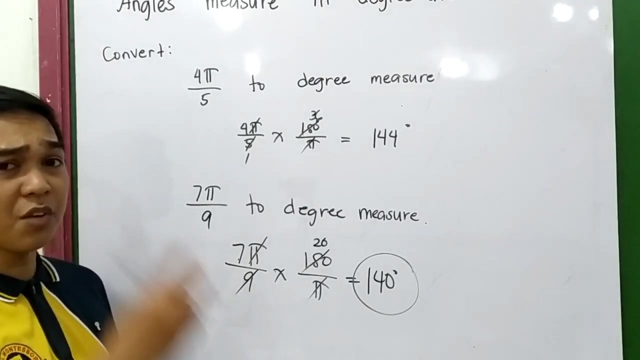 If our angle rotates counterclockwise direction, then the measure is positive, And if the angle rotates clockwise direction, the angle is negative. We also have the con-terminal angle. Con-terminal angle, two different angles with the same initial sign and terminal sign. 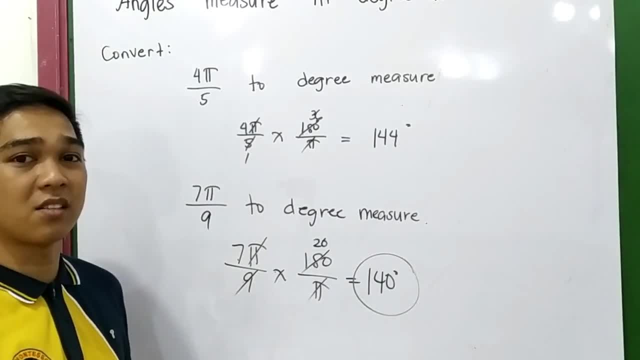 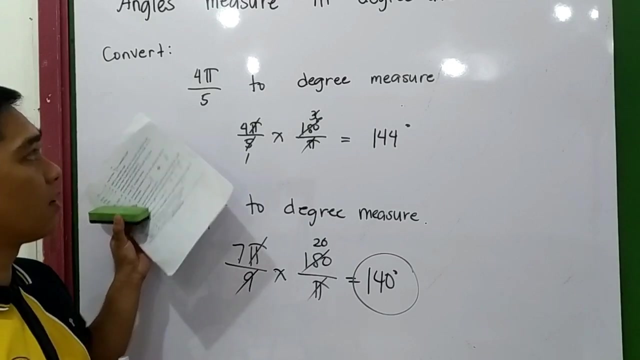 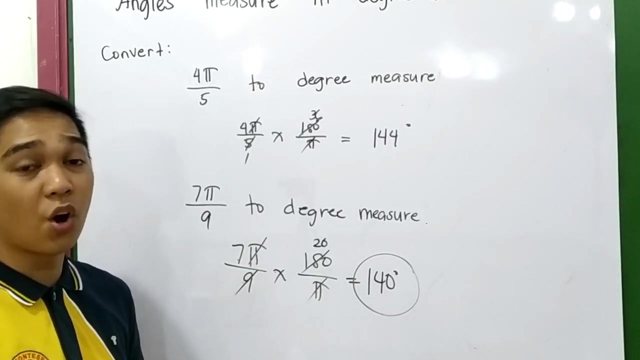 Quadrangle angles are angles that lies in x-axis or y-axis, or simply the multiples of 90 degrees, And angles measured in degrees. If they ask you to convert degree to region, multiply your answer into pi over 180.. And if they ask you to convert region to degrees, multiply 180 over pi. 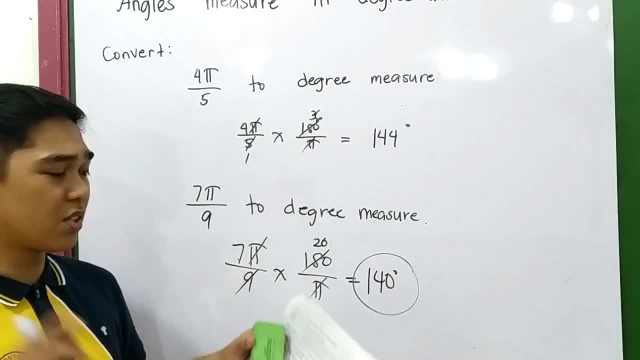 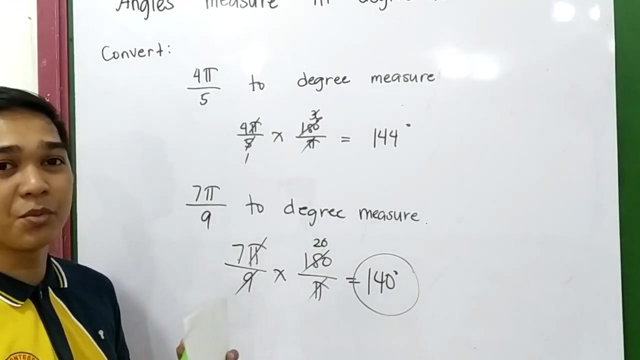 So thank you for watching and practice more, because this is the introduction of trigonometry, So it is fun. It is very hard to explain this topic, So I hope you learned something for this lesson and start practicing. Practice in your handbook. search in the internet for more information. 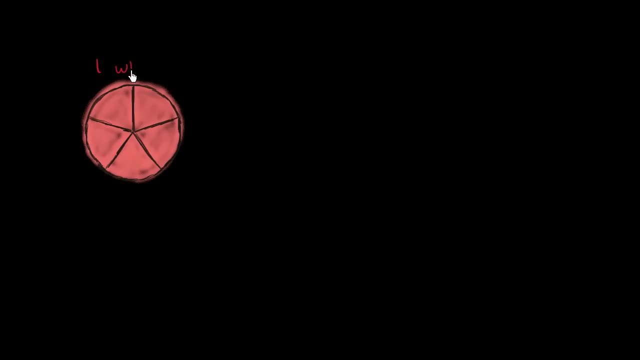 Let's say that this circle right over here represents one, one whole, And we've divided this circle into one, two, three, four, five equal sections. So each of these sections represents one-fifth. Each of these sections represents one-fifth of the circle. 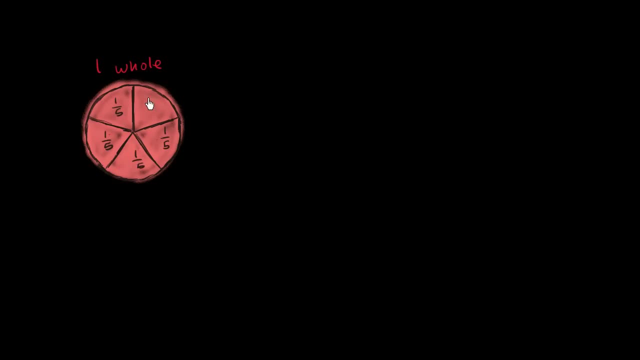 We've seen this already One-fifth, one-fifth, one-fifth and one-fifth. And if we were to then color in some of this? so let's say we were coloring three of these sections, So that's one of the sections right over there. 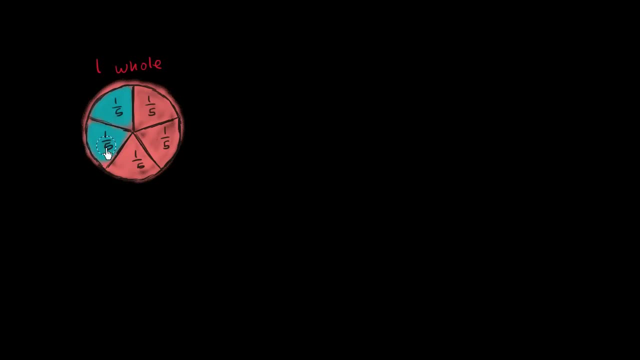 another one right over here. So we've colored in two of the fifths and then three of the fifths. Notice you put those three one-fifths together. how much have we now shaded in? We've shaded in three-fifths of the whole. 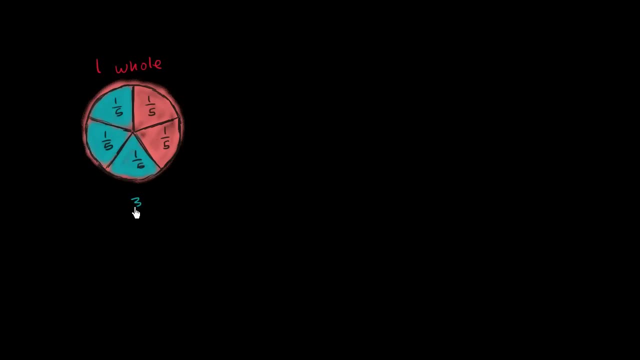 So the fraction that's actually shaded in now is three-fifths. Three-fifths is what's shaded in Now. let's do this. Let's do something in some ways a little bit simpler, but also in some ways, kind of interesting. 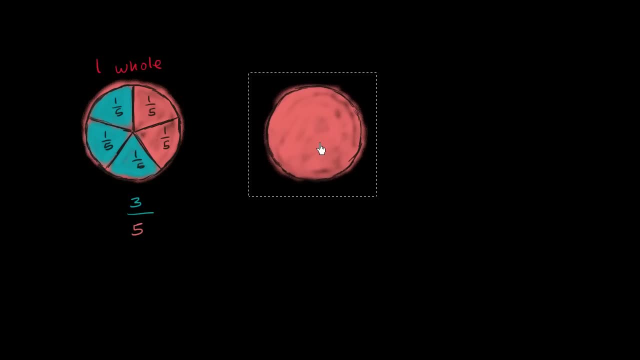 Let's start with a hole again. So, once again, this is one hole. Let me label it one hole. So it's one hole, And instead of dividing it into five equal sections, I'm just going to divide it into one equal section.